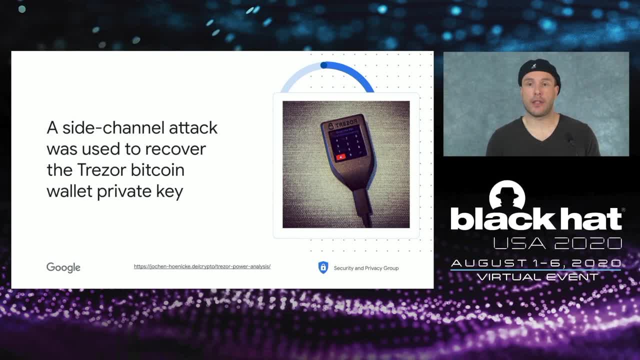 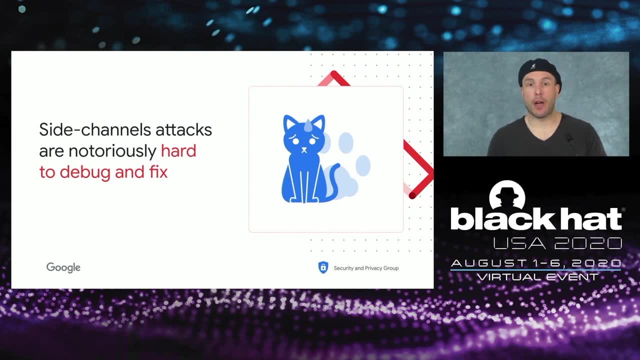 be and how devastating having a side-channel attack can be for secure hardware. One of the problems when you develop software and when you develop hardware- when you develop hardware compared to software- that debugging it is harder because we have to find where the session attack came from, which. 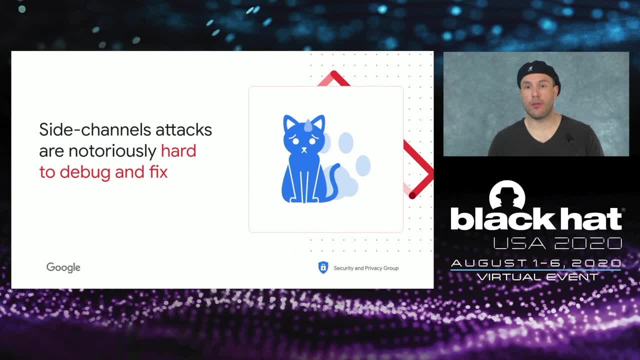 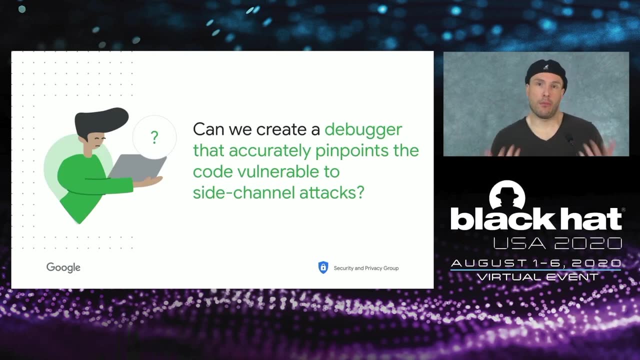 means where is the leak into? into the code, and this leak is usually due to the interplay between the software and the hardware, and so you have to look at both of them at the same time to get an idea of what might be leaking. this is what make it so hard. so if we were to have a more secure 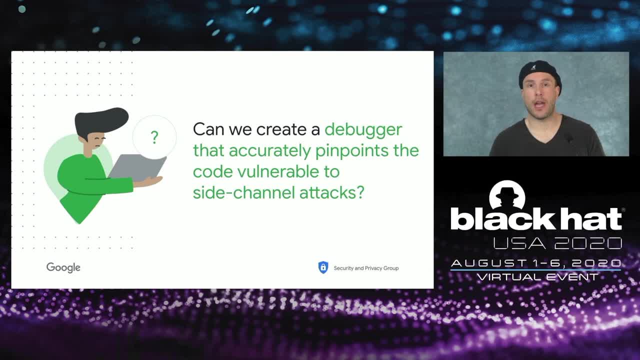 or the most secure hardware possible. we need to help reduce the cost of finding the attack and being able to pinpoint them accurately. this is why we asked the question: is there a way to create a debugger that will help us to pinpoint accurately and quickly? what is the part of the code which 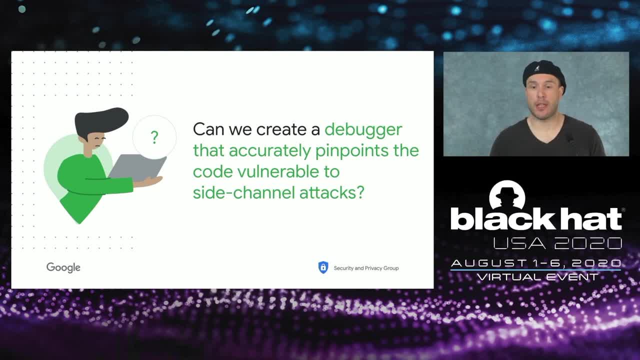 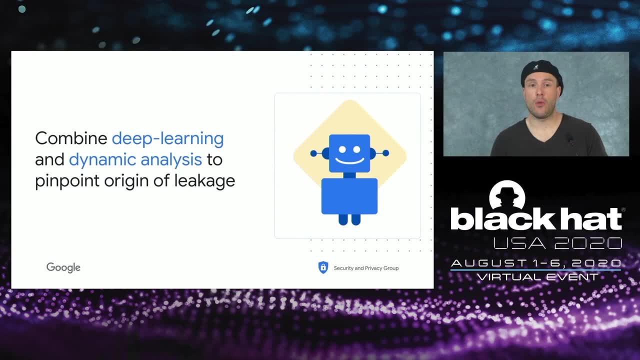 is interacting in a way with the hardware which make it vulnerable to side channel attacks? and the answer is yes. we do believe that, by combining deep learning and dynamic analysis, we'll be able to quickly and effectively find the pinpoint and quickly find the origin of the leakage right, the leakage being 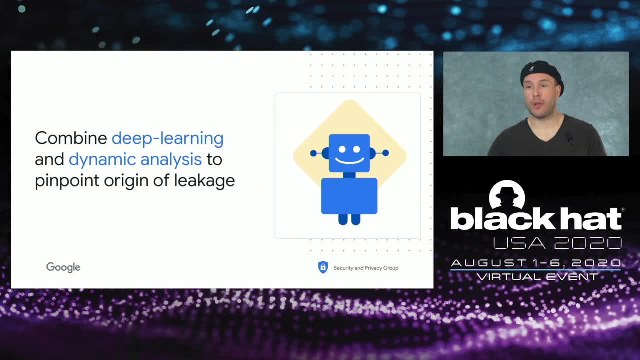 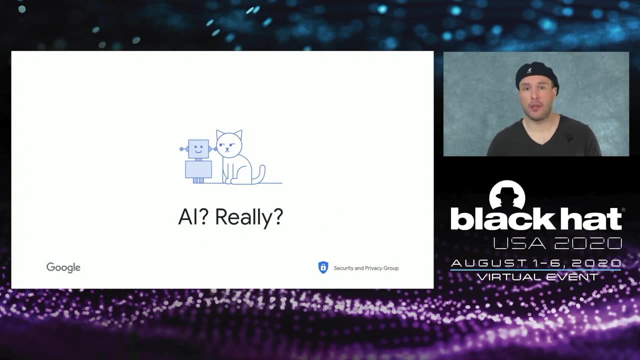 where is the implementation, is giving information that can be used to extract the key and, of course, because i use the word deep learning, you might be a little bit skeptical and say, well, yet another talk about deep learning, machine learning. i'm going to sell you something. the truth is, why not we actually? what i'm going to do today is actually show you. 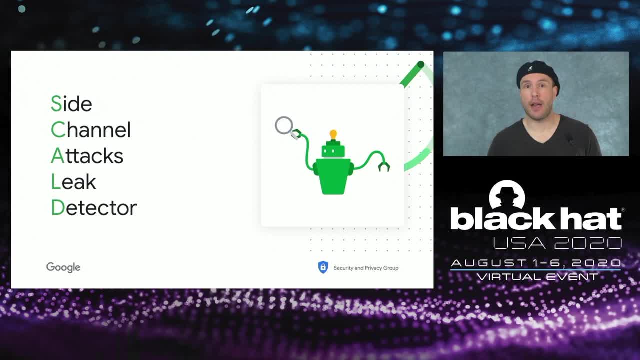 a early prototype of a concrete software that we have developed, called cold, which stands for charge side channel attack leak detector, which is actually is able in practice to help us find where the leakage come from and help us debug side channel attacks. so, to make it very concrete, today what we're going to do is 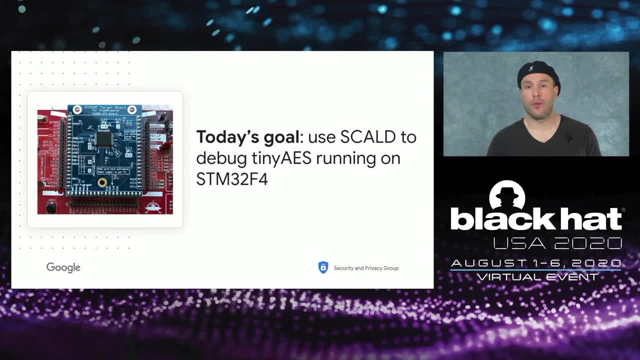 we're going to show. i'm going to show you how we can use cold to find where a tiny irs implementation running on an smt32 f4 is leaking. and this is a very, very, very, very, very obviously a unprotected implementation tiny irs which is running on a well-known arm cp. 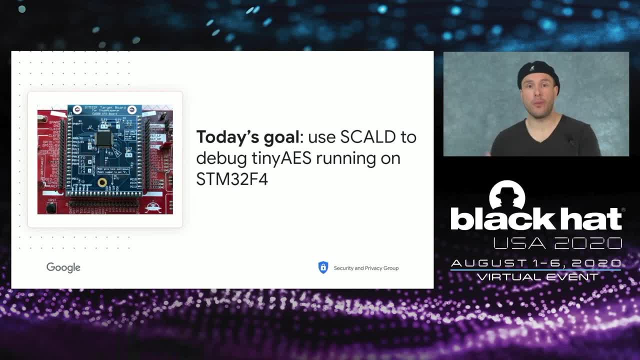 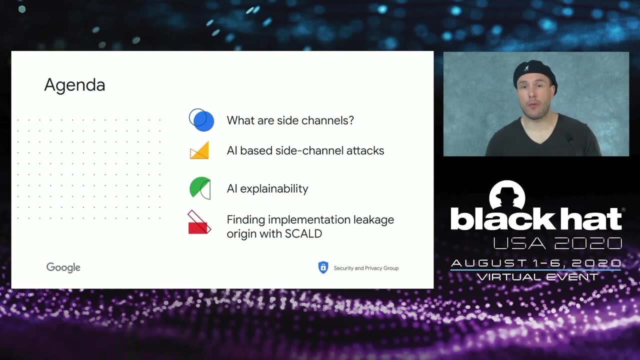 and this combination of tiny irs and smt32 is what we call a target, because, as i said, the side channel attack is due to the interplay between the implementation and the hardware. so how are we going to get there? first, i'm going to briefly recap what side channel attacks are. 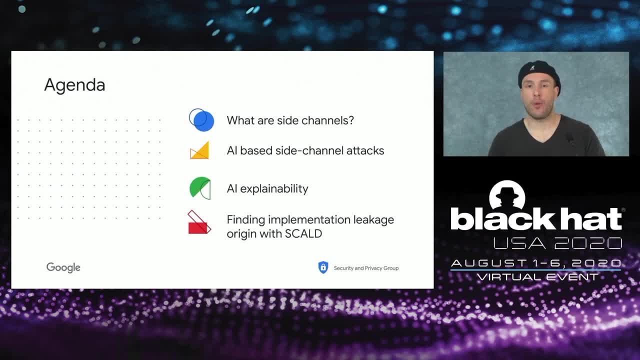 then i'm going to tell you how we very briefly, how we perform side channel attack, which are using an ai, deep learning, which is what we presented last year. then we're going to talk about a explainability, which is a core of the technique we are leveraging to do the debugger. and finally, i'm going to show you how, in practice, we we use 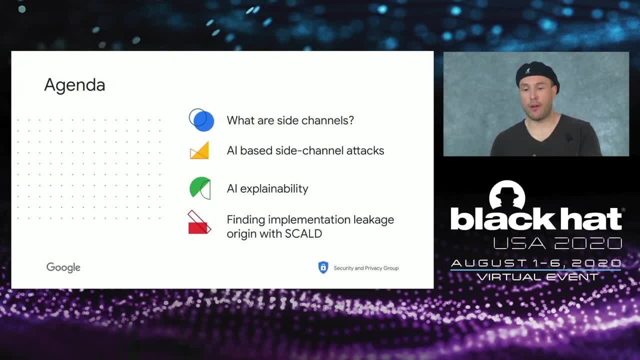 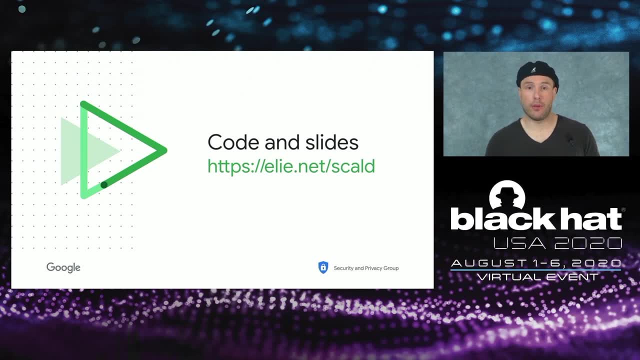 it to find uh leakage into our target. so if you want to follow along at home and you want to look at where is the, where the code and the sliders- we call the sliders- we call the sliders and when you go through the presentation you can get them at elinet slash code. 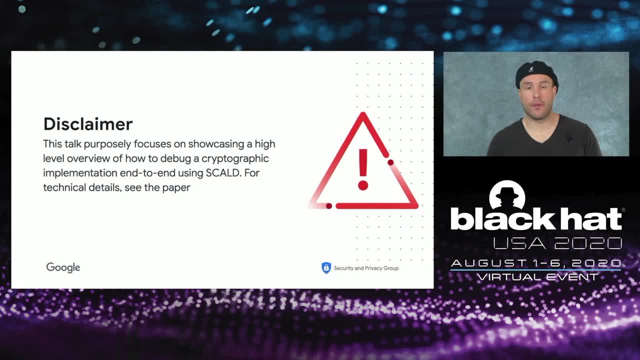 a quick disclaimer about this talk. the goal of this talk is to provide a high level overview of how the whole thing works and provide you an end-to-end view of how the process works. if you're interested in more technical detail, like the exact machine learning architecture we use or 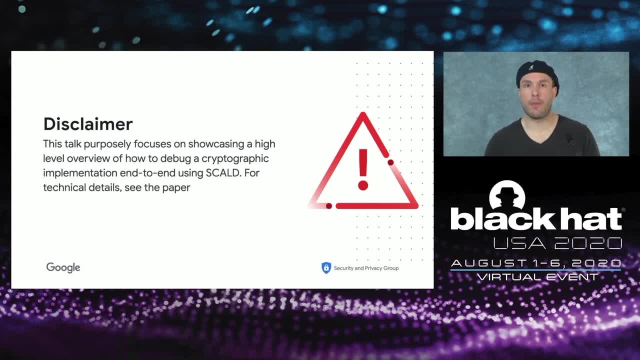 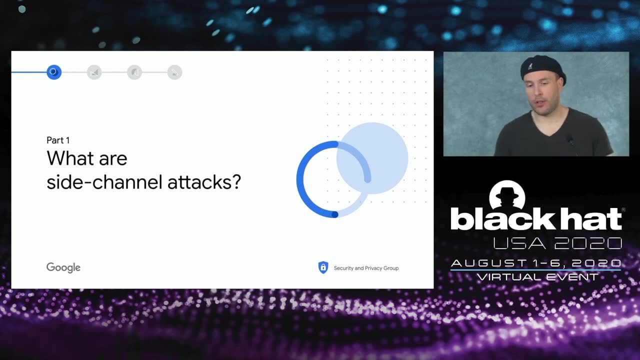 how we do the code mapping and everything, uh, which you should have by the time of black hat a, you can read, and we will provide you all the detail as well as code, who enable reproducibility. so, with that in mind, let's start by what our channel session attacks. so everyone is on the 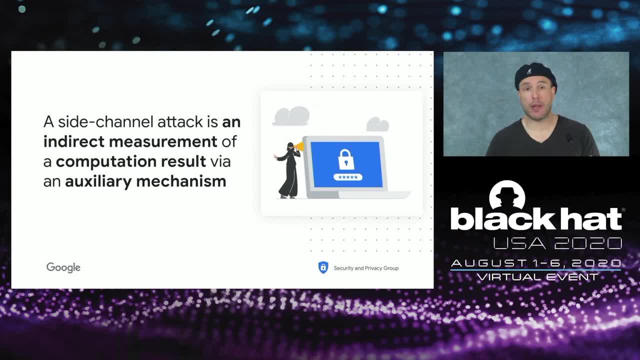 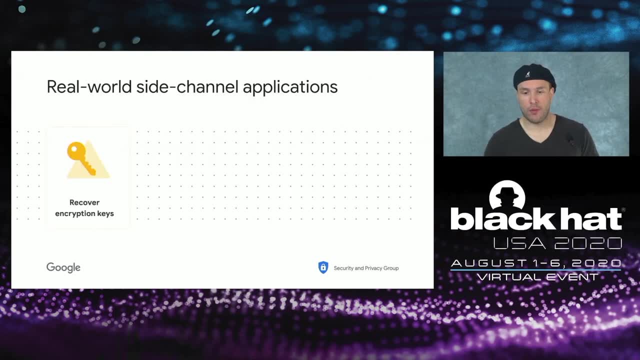 same page. a session attack is basically an indirect measurement of a computation result, which is done through a auxiliary mechanism. so what do we mean by that? well, sorry, before getting there, let's, but what is? why is it useful where a side channel attack is used, as i mentioned, and 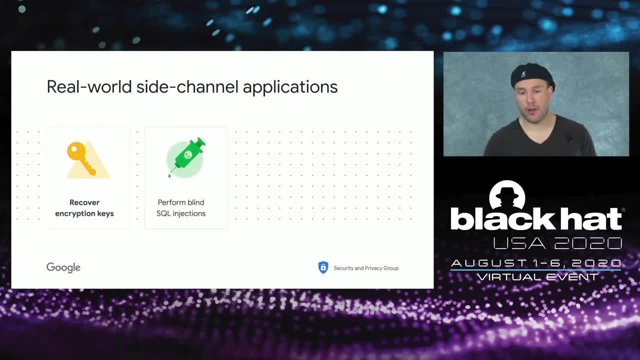 the intro, to recover encryption key. it is also used in the world of web security to perform blindness injection, where you cannot see the result of the injection, so you have to guess what is the result. it's also used to tilt password and pins. and finally, it can also be used to 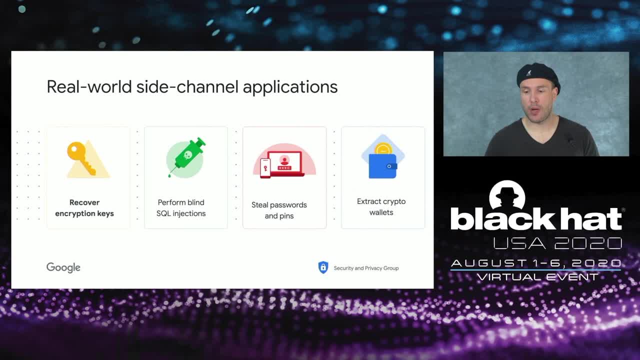 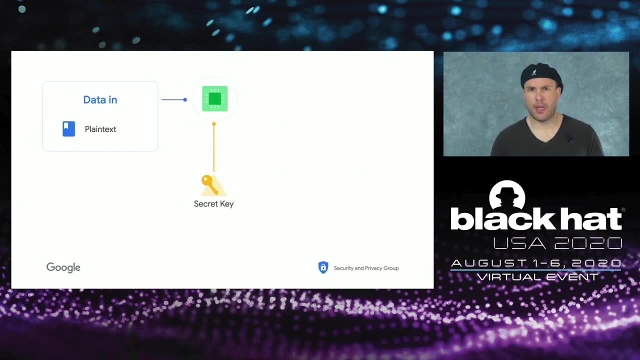 extract, as we showed in the example earlier, extract crypto wallet private keys. so basically, everything which is secret that you cannot observe directly but you wish to guess or to recover, can usually be detected by a session and attack one one another. so in the case we are interested in, which is 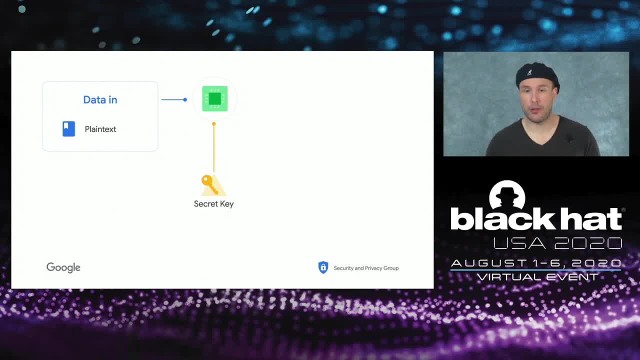 hardware crypto. the idea is, when you perform a computation on a cpu using an algorithm, you feed in your data, which is your plain text and your secret key, and then, as a result, you obviously get the encrypted text, but you also get a bunch of leakage. so leakage, basically, are this kind of 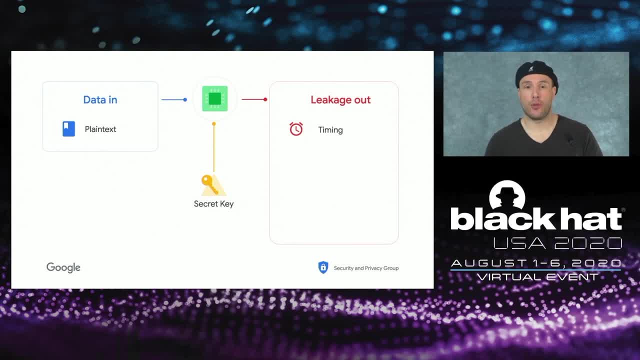 side effect on internet, side effects which are due to the algorithm running on your target. so, for example, the algorithm will take some times and unless your algorithm is protected against timing and is constant time, you will see different type time- execution time- based on the input. similarly, and that's the one we're going to focus on during 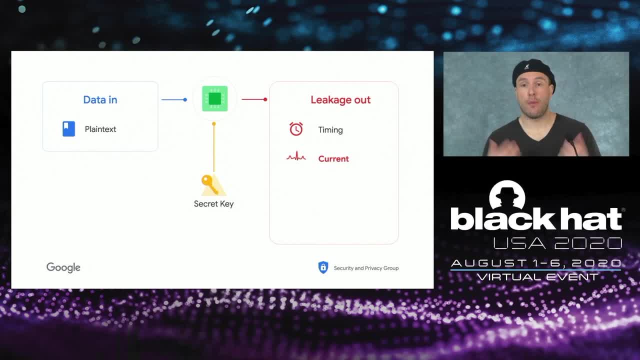 this talk, you might have leakage which are due to power consumption. so depending on what operation is done, you get different type of power consumption and you can actually extract that. similarly, depending on how powerful some part of the cpu might hit differently. this is not really used for recovering hardware crypto. 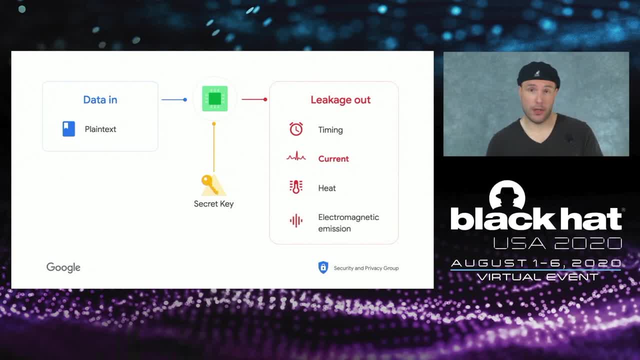 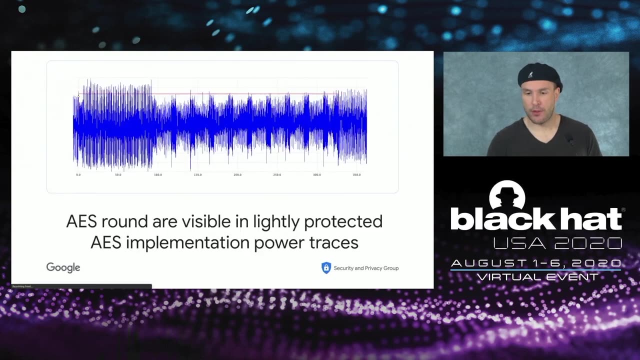 in our case, but this is something which do happen. and finally, least last but not least, sorry, the. you have em, electronic magnetic emission, which is also very powerful, and it is the other way to one of the other way you can extract and recover a key. so here's an. 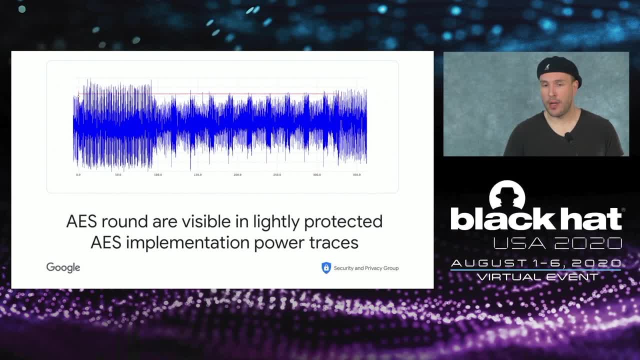 example, for power tries, because that is the goal of our talk. as you can see, this is a power trace which was captured, uh, during execution of as, and if you look closely in the middle, you will see that you have 10 spikes. it turns out that each of those spike is actually describing or is actually representing a 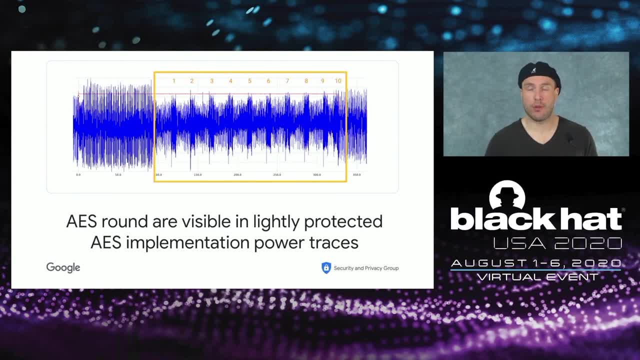 as round right, there is 10 rounds for as 120, 128, and we can see very clearly on the trace that those rounds are visible. if they are visible, then they might contain information. if they contain information, we might be able to exploit it to recover the key. that is what a such 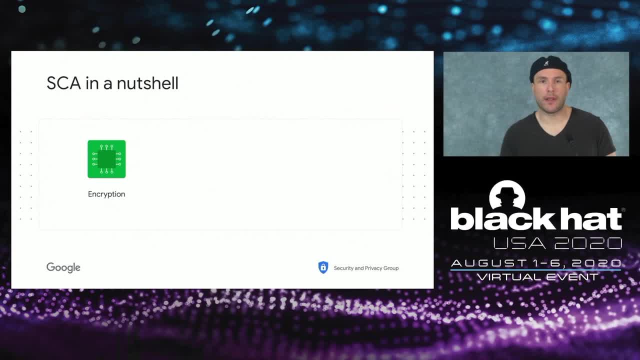 attack is. so to further that a little bit more, what happened is the cpu. the cpu computes the encryption, and what we do is we measure the current with an oscilloscope and then we, in the traditional setting of such an attack, you perform something like a template attack, which is you: 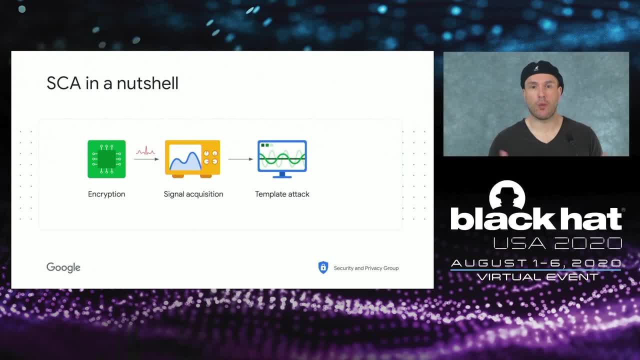 take all the traces collected. you collect a few of them- actually you don't collect one- and then you combine them statically to try to pinpoint what is your current attack, as a conspiracy under which you do sort of analyze, and to calculate what is the current current. 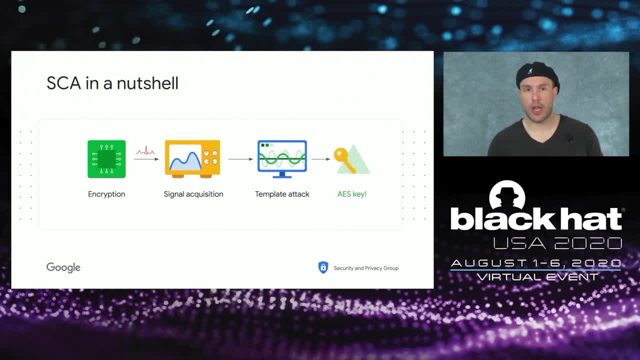 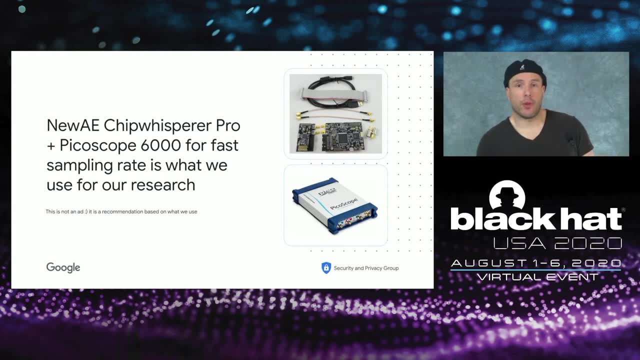 key value and then you recover the key. That is, you do not share what the side-channel attack is In our research. because we got the question asked a lot: what do we use? We use a new AI, CheapWhisperer Pro, and we sometimes use a Picoscope 6000 when we need faster sampling rate. 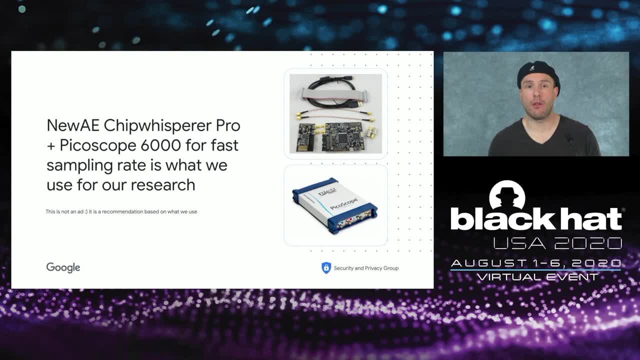 depending on the target. In this talk it has been said we only used the CheapWhisperer Pro to do the capture of the trace because we are going to use synchronous traces for only the first few rounds. When we do as-previous work, the whole trace is for the whole implementation and we want 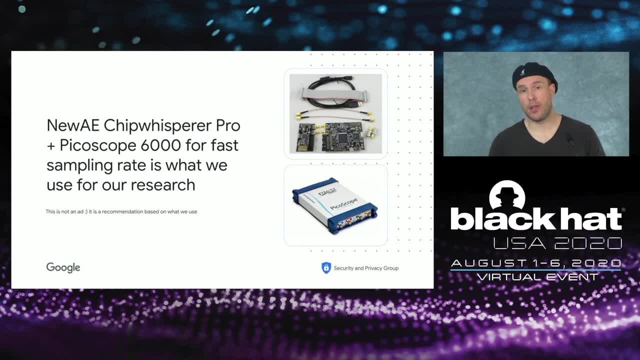 to do it in the attacker settings, where we don't have the clock. We use also the Picoscope. Again, this is not an endorsement for a product or another. it is just that this is what we use in our lab. So if you would like to reproduce our results from the ground-up, this is what you could use. 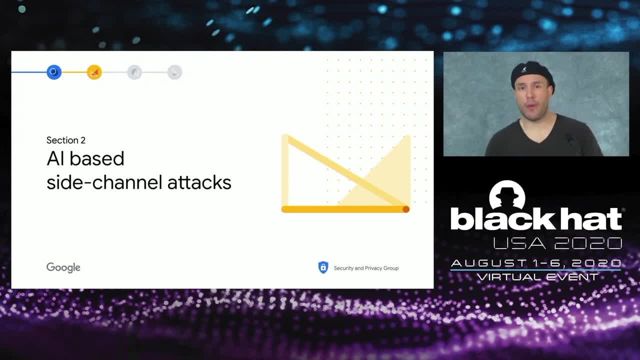 So let me now describe a little bit more of how we wave in deep learning, because we are going to need the machine learning model generated during the attack for the debugging. So deep learning, side-channel attack. we call them side-channel attack, automated with machine learning. 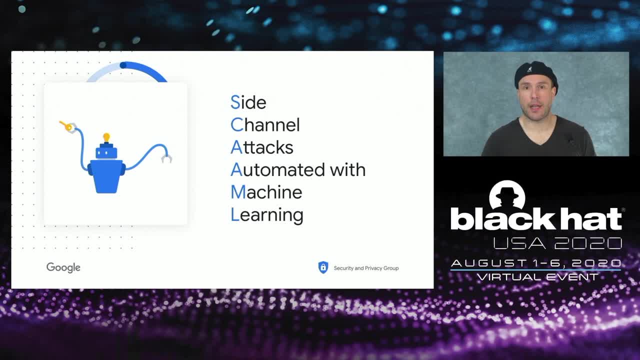 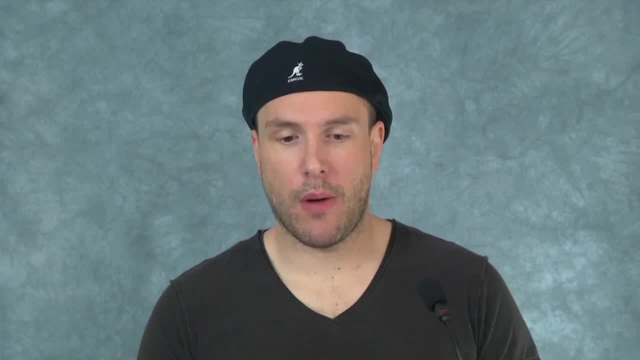 and the idea is you are going to replace the template attack with something else, with a neural network, and this is something we have covered in detail before. However, I am going to briefly recap today how you can do those attacks in practice, so you are able to figure out, to get a gist of. 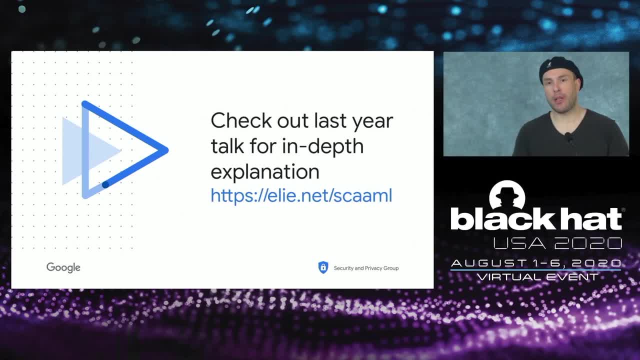 what is happening. If you would like to have a more in-depth explanation of how the whole thing works, we had a talk last year at DEF CON where we actually got into greater detail for 40 minutes on exactly how that works and all the nitty-gritty 10 bits, and you also have the code associated. 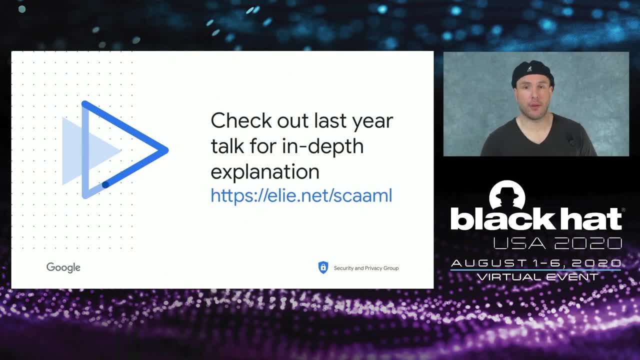 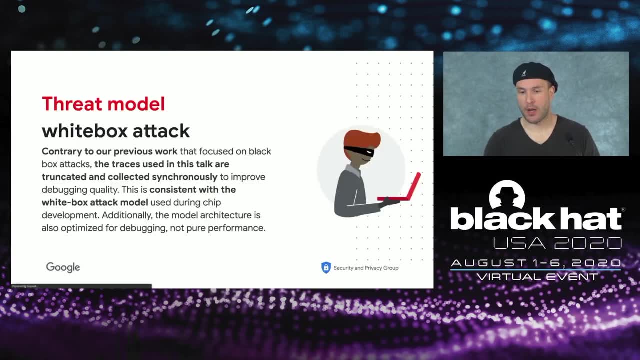 with it. So if you want to go there, you can just get a slide and the recording of last year's video at that address. All right, One thing which is different from last year and which is different from our threat model, where we try to do a black box attack, which is the strongest thing we can do. 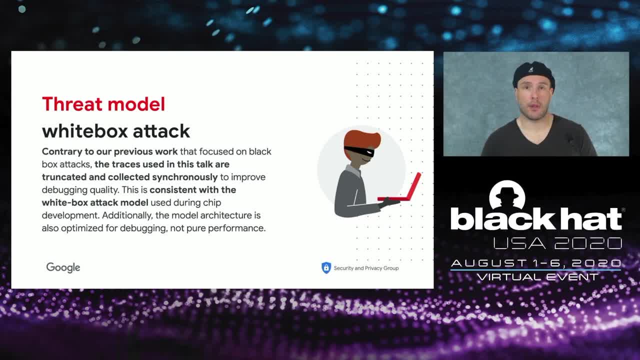 when we try to revise the security of a chip. in that specific case, we are building a debugger, So we are building a tool which is for the people who built the hardware or are not necessarily building the hardware but are creating the secure token. So we are taking a white box attack. 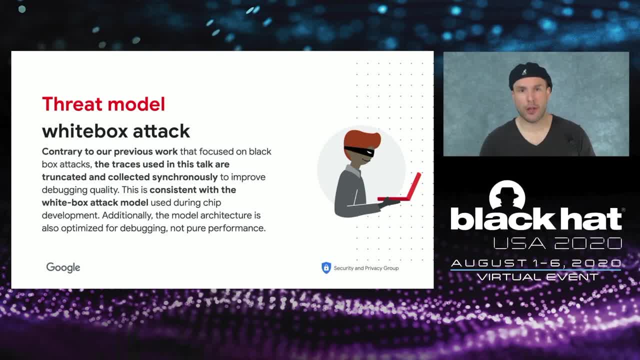 which is, we have access to the source code, we have access to the clock and we have access to knowledge about the implementation. As a result, we are simplifying the attack by using synchronous capture, which means we are using the internal clock of the target. 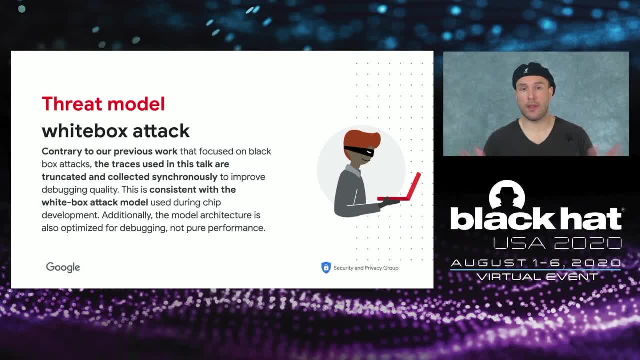 to capture the trace. It makes it easier because we have traces which are perfectly aligned, which you don't have in a black box settings. We also are reducing the amount of points in the trace that we are capturing, because well we know that we only need the first round. 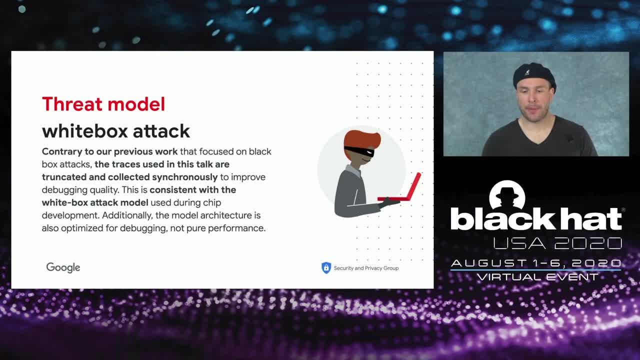 the first round and a half or something like that. So that makes it easier for us to train the model, because of course the trace is slower, is smaller and we are aligned. so the model has to do less work. so we can use smaller models and also it converges faster, It's easier, You could. 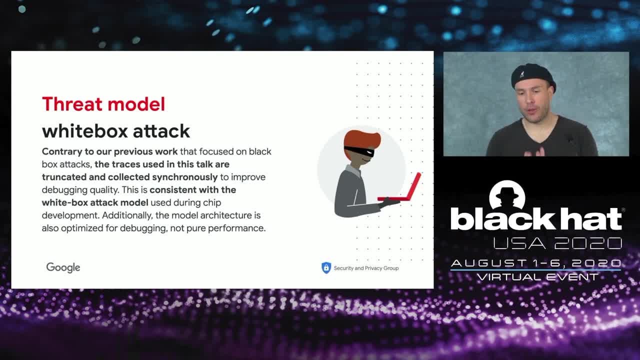 do it with the full scale model if you wish, although it's going to create a lot of dead space, which is not necessarily useful for this type of stuff, as we want to do it with a lot of other stuff, as we want to have as quick of an interaction as we can. This is why it's a white box model. 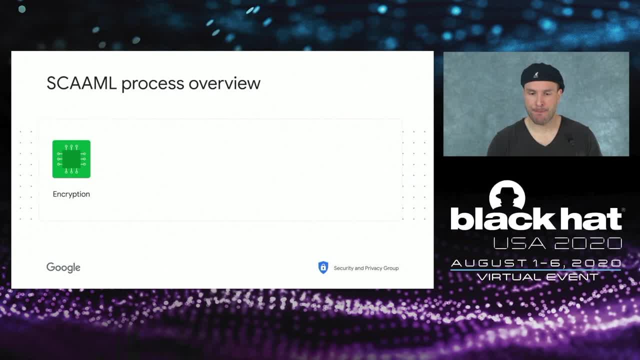 This is why we did choose the white box model. Okay, So how this camera process differs from the SCA processes that we saw earlier. Well, we start with the template, which is you perform. Second, my Google Assistant decided to carry over. 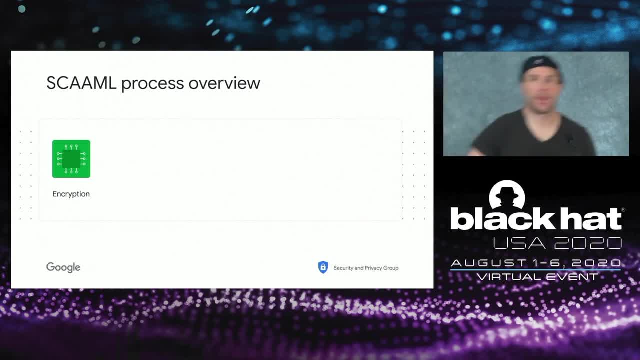 Sorry about that, Unexpected during, But given the condition, the phone is not just here, All right. So let's go back to where we were. So we have the encryption and then the encryptions basically will happen, is the encryption is performed as usual and then we capture the signal. 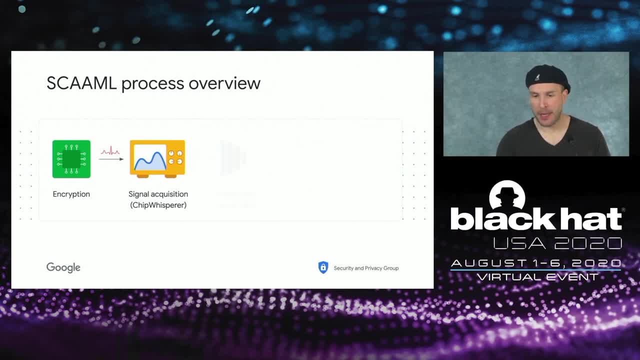 with a cheap whisper right, and then we get a bunch of traces And then, instead of doing the template attack, what we do is we feed those to a deep neural network, which is deep learning, a form of AI, and then the machine learning is going to make a prediction. 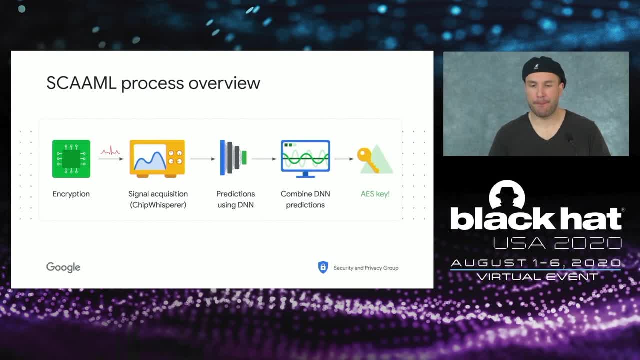 and we're going to combine them to recover the key, And that's what it does. The advantage of this technique is it's fairly automated, doesn't require too much domain expertise and also can work on very complicated targets quite efficiently. As I said, it works really well in black box settings on the full traces. 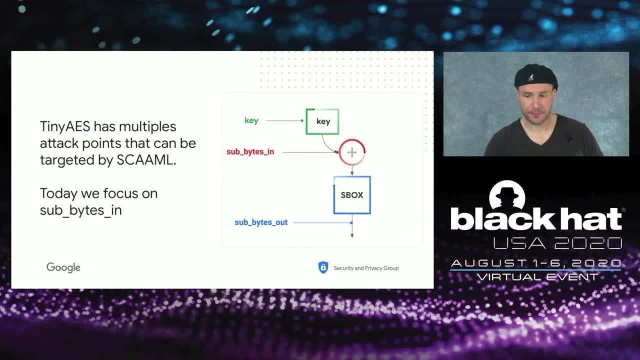 which is something that all the type of approach struggle with. When you do targeting, by the way, when you do target an implementation, you might try to target directly recovering the key, but more often than not, we try to target what we call intermediate. 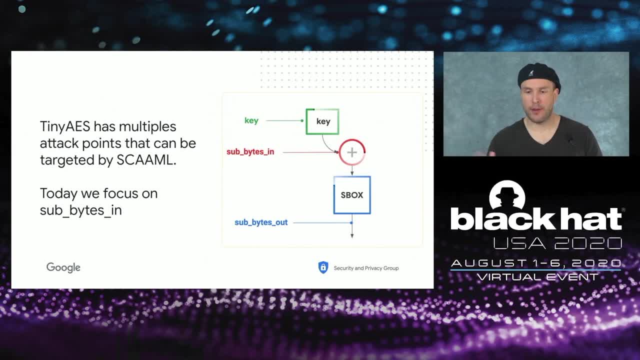 which are part of the AS. part of the AS where there is some sort of memory loading or memory unloading, because this is where the power is going to be stored. So the power is changing right because you are setting some bytes to one. 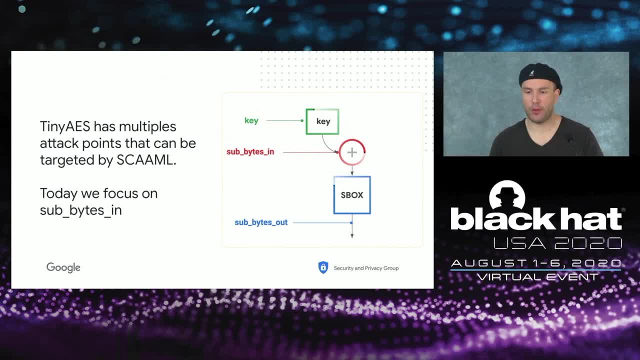 some bytes you are putting to zero, so the power is changing right. So we want to have this kind of point. Those points are called intermediate points. There are quite a few of them, The three canonical ones that most people use, including us. 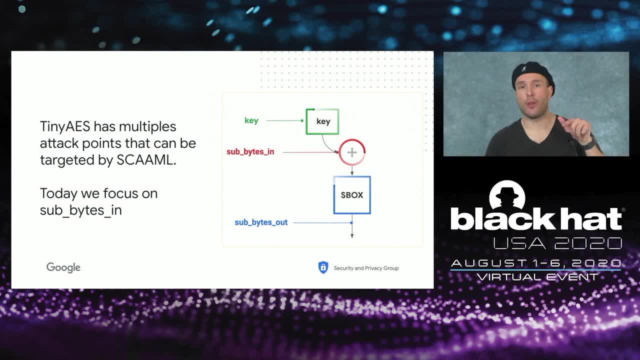 are the first initial three which are part of the initial round of AS, because they are easily invertible, which means you can directly recover the key from them. Today, we're going to only focus on one of them, which is subbyte in. 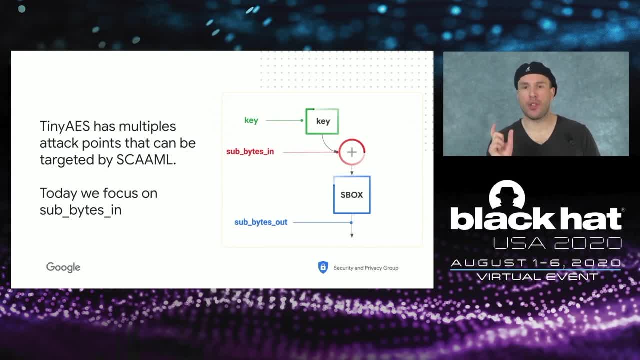 Which is basically the intermediate point which happened, as you can see on the diagram, after we have XORed the key with the plaintext, You could target, also subbyte out if you wish. As we explained earlier in the previous talk, trying to target the key doesn't work really well. 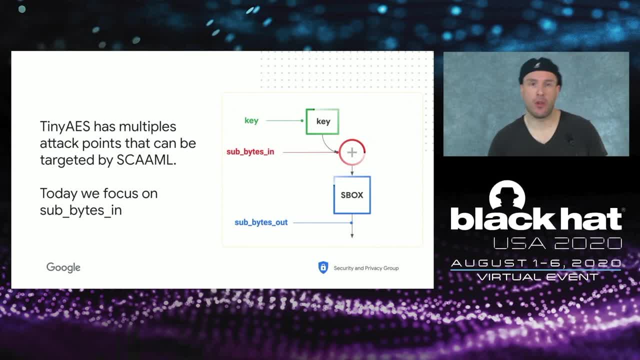 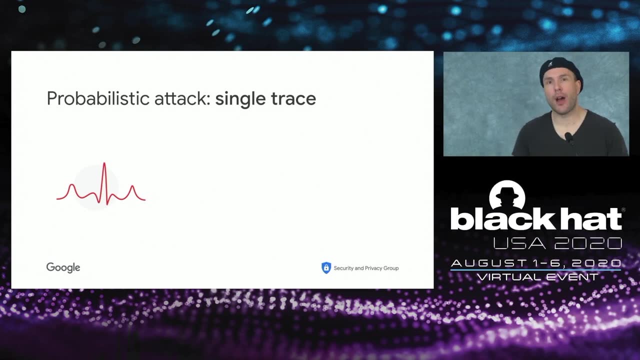 This is not a vulnerable point for tiny AS, so your model would probably not get as good of an accuracy And given that we are trying to get for the most obvious leakage for now, subbyte in is perfectly fine, Okay. Last thing I want to mention before we move on to how to do the debugging is: 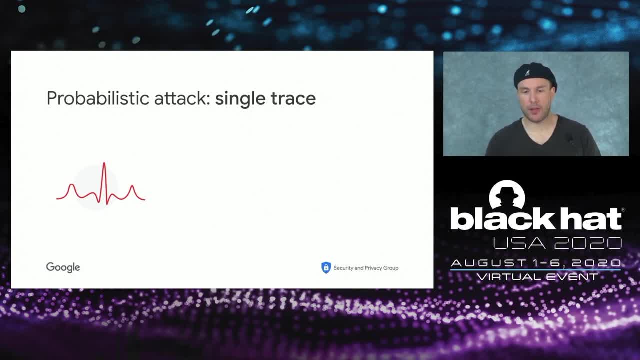 what do you do with a prediction? Because that's one of the nice things about machine learning when you do deep learning based SCA, is that you get your traces and then the model, instead of telling you one value, would give you a probability. 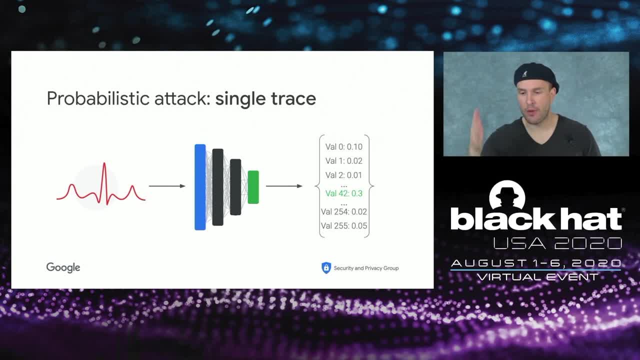 a fake probability, but a probability to the softmax would tell you, for each value of the intermediate, what is the probability or how strongly he believes each of them is a correct prediction. So what you can do is give rise to a very natural probabilistic attack. 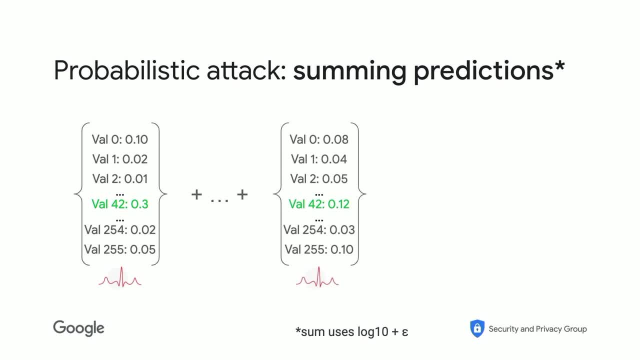 where, basically, you take all the output of the model. so the model would tell you for each value, potential value, what is the probability. so you can actually sum them using a log10 plus epsilon and then you get a distribution And that helps you to accumulate probability very easily. 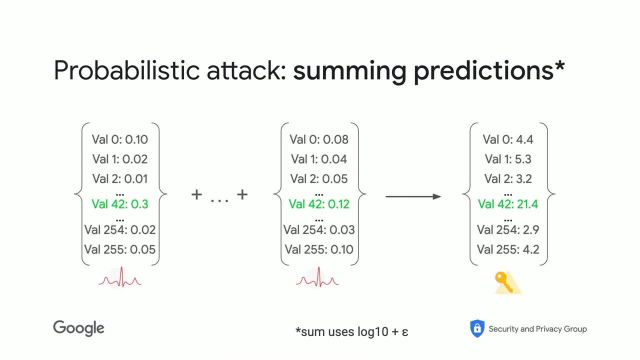 and tell you which is the first guess, which is the second guess, third guess, and you can actually rank your guess, and so it makes a very nice probabilistic attack that only deep learning provides. So that's also one of the benefits of using deep learning based SCA. 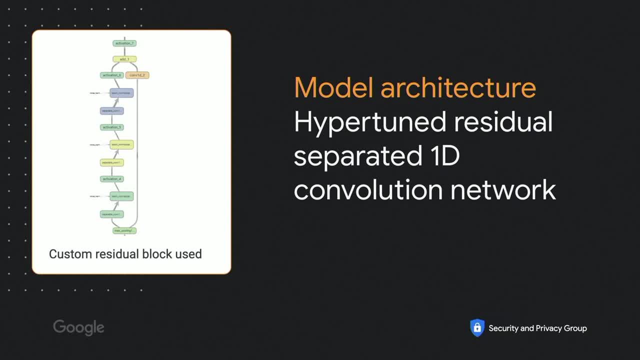 In this current. to give you a little bit more detail, the model we're going to use in this talk is something called a simple hyper-tuned, residual, separated, 1D convolutional network. Basically, what it means is we use 1D convolution. 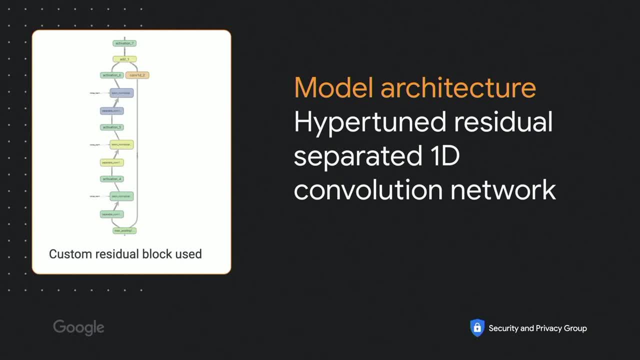 We use separated 1D because they are faster and have less parameters and in our experience over the last three years, it feels that it's good enough. It actually gives us performances, It is able to work and converge, so we don't need the full convolutions. 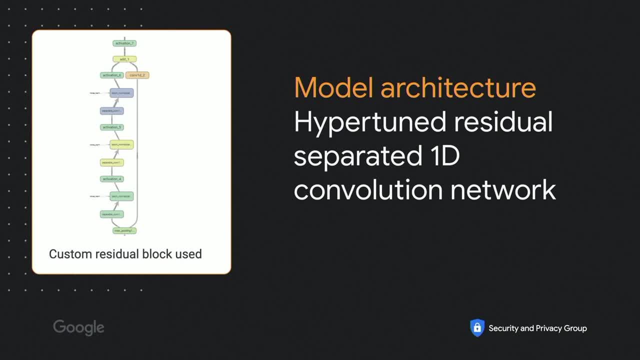 We also have hyper-tuned them before, so we basically use one of our best models. And then it's a convolutional network, which means it's mostly based on convolution, And the residual part means that we tend to do something like the ResNet implementation. 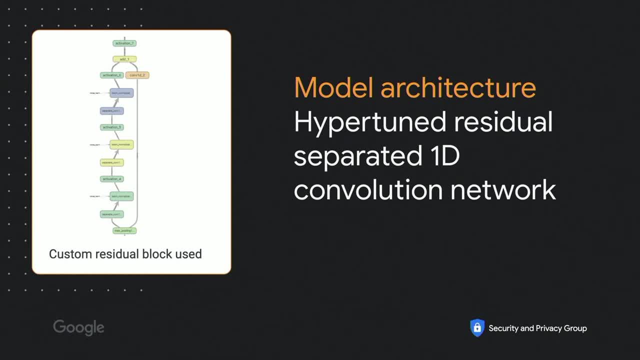 which is basically we do a bunch of convolution and then we keep the signal by having a second path that you can see on the right side of the diagram, which helps us to maintain the flow of the gradient and avoid vanishing gradient problems. So again, it's very standard. 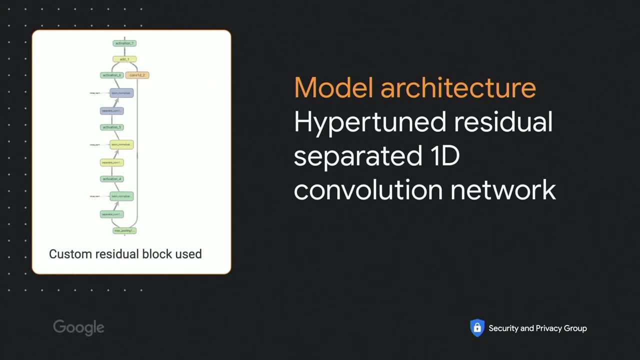 If you do machine learning, it's just adapted to work well for 1D traces and you can construct your block differently. It seems that this block is the one which works best for us and basically we stack a lot of them like pancakes. 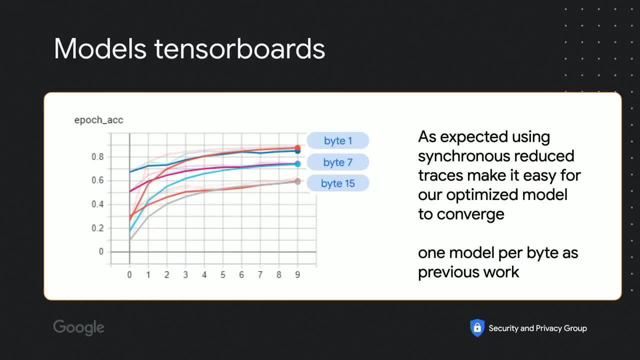 which is why it's called deep learning. Here is an example of what you might get if you train this model. We have three models which are trained. because we train three models for this talk In the real setting, you will train 16 of those, obviously. 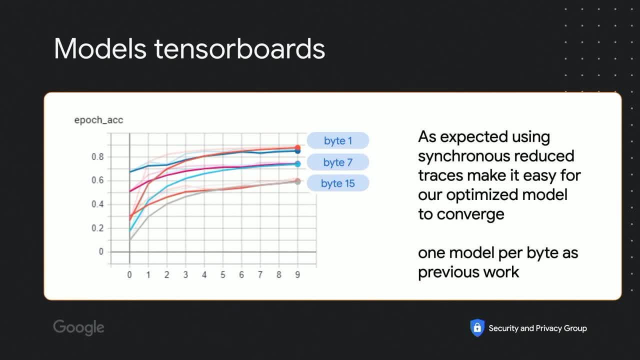 And what happens is basically you can see those three bytes converge very well after only 10 epochs. We could have kept going to increase accuracy, but at that point each model has reached above 60%, which is plenty for what we try to do. 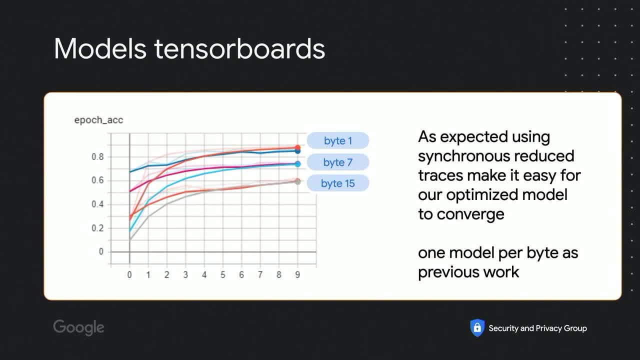 which is get a bunch of traces where the model is able to predict the correct value and then use that to debug. So that's plenty enough. So we stop there, because obviously we want to be as efficient as possible. As you can see, the important part here is: 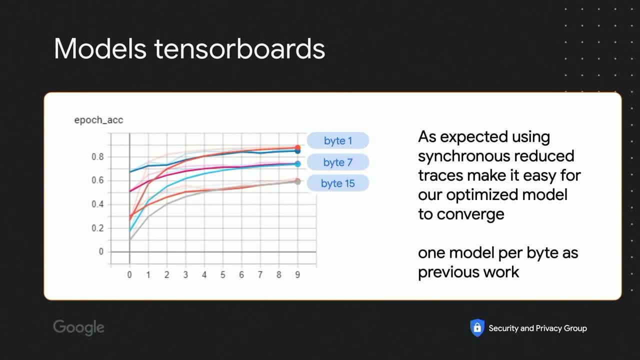 you can see that the validation- so there is two curves for each of the points- is actually tracking very closely the training set And that's really good, which means the model has generalized perfectly because both are tracking each other. So we have a model which generalizes well. 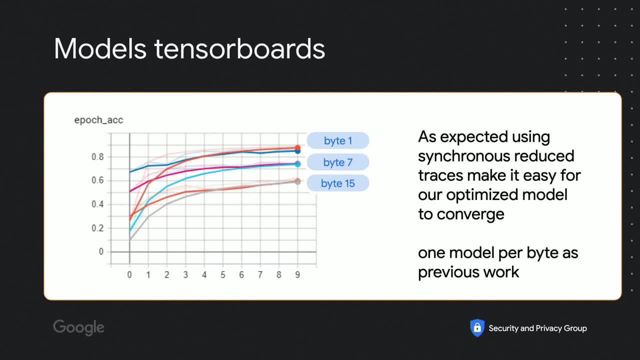 So that's a good model. Again, that is expected because we made it very easy for ourselves by having an unprotected implementation, tiny errors and make it synchronous, and shrinking down those traces to only the first 4,000 points. So that's what it is. 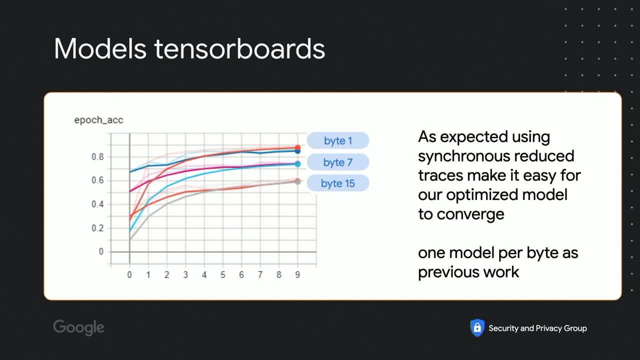 Last but not least, as I mentioned on the side, if you're not familiar with how session attack works, we do tend to recover one byte at a time, So you need to recover the whole key 16 models and then combine the prediction to recover the whole key. 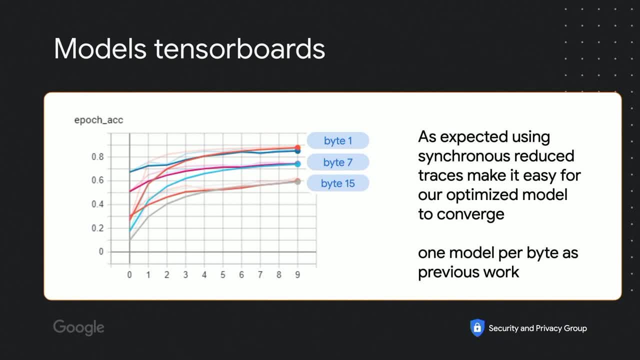 For the rest of the talk. I'm going to only focus on one byte at a time, because you basically repeat the same thing 16 times. I'll show you some example of how the debugging looks like, different from both traces for different bytes. So keep in mind that we have multiple models. 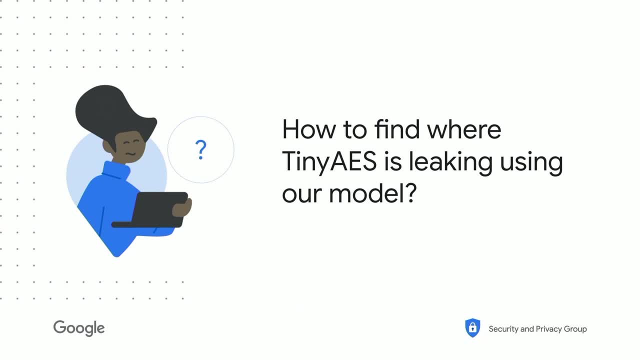 Okay, So now we have a model and we know our model is efficiently breaking tiny errors, So the implementation is broken very, very badly. So, okay, can we use that now to figure out where the leakage is coming from? Well, yes, 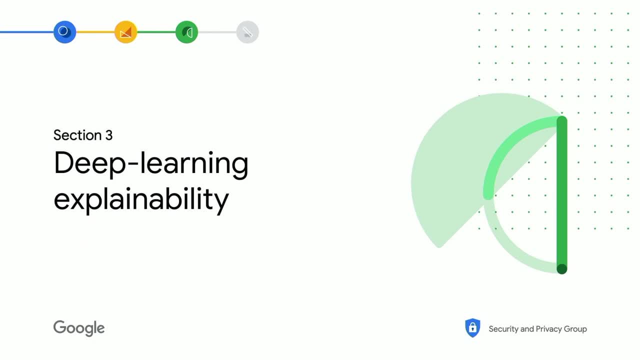 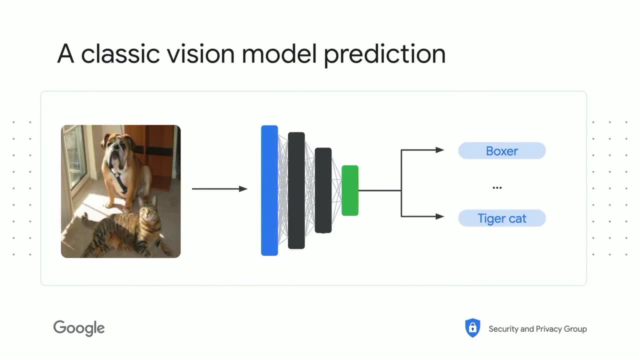 To do that, we're going to leverage a known technique, a known set of techniques actually, which is deep learning explainability. Deep learning explainability actually was developed for a vision, As I already said, early stages, So they had a bunch of data sets. 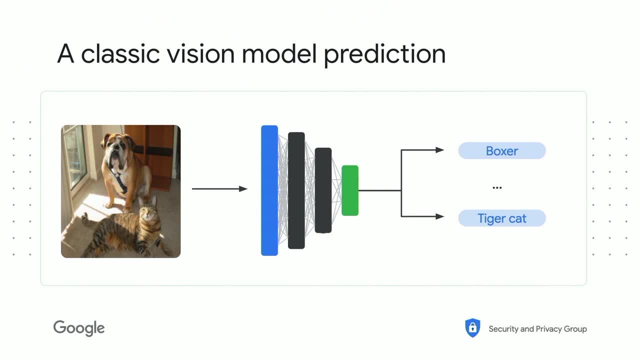 And the model, for example, will accurately predict in this image that it contains a boxer and a tiger cat. The question is why? What is the policy image that the machine learning is using to decide whether there is a boxer or there is a tiger cat? 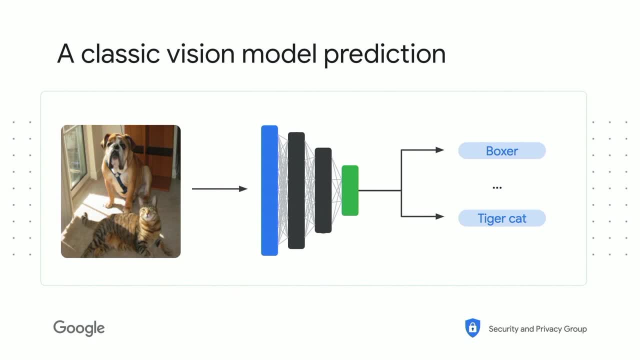 You want to use that to make sure there is no biases or errors into your data set that are giving hint to the machine learning that it should not pick up. and it did generalize correctly, right? You want the machine learning to not only detect a cat in that image. 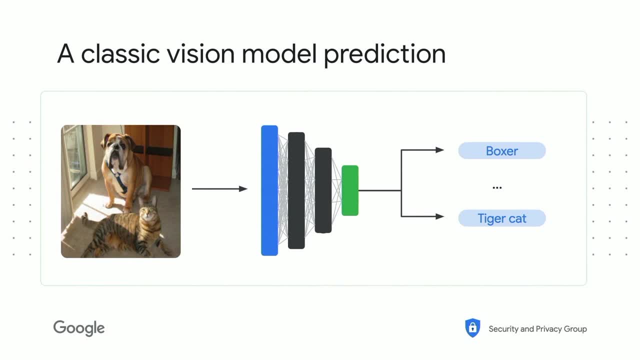 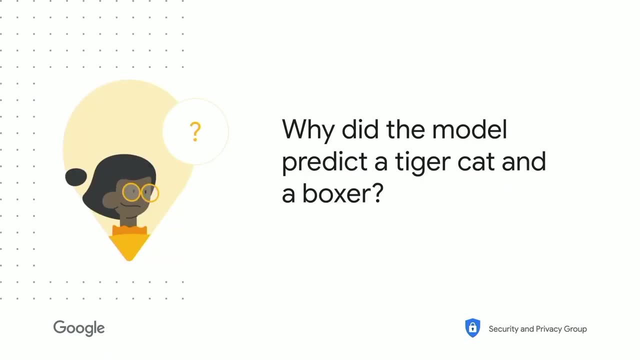 but also detect it in any wide range of images. So you want to make sure it focuses its attention to the right place of the image. So the way you do this is, as I said, to answer that question, the way you do this is you use an explainer technique. 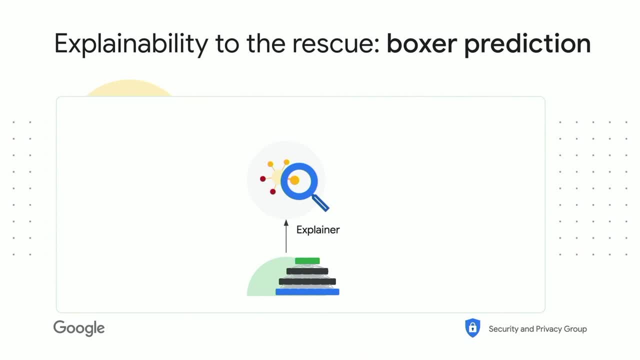 There are a few of them. I'm going to highlight a few of them after that. And so basically, what you do is you feed to the explainer the model, You also feed the image, And then you ask it why this class was predicted. 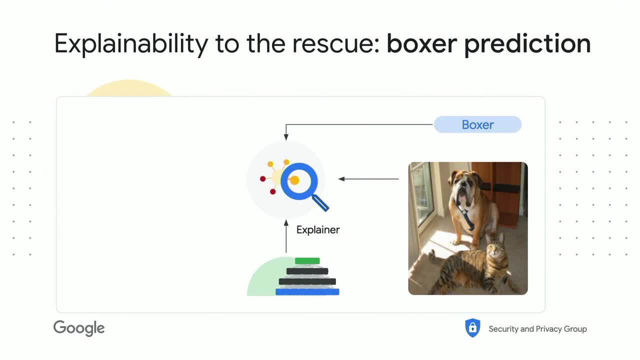 You can ask the main classes, or you can ask a class which is not the main one. You can decide which one you want. But basically what you're doing is you are conditioning the explanation based of the prediction you want to explain. So you basically provide the input and the output. 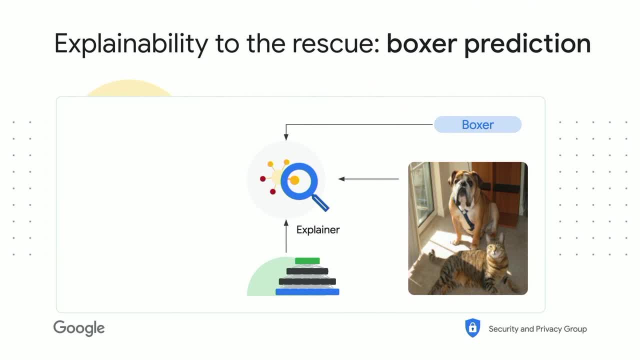 In a way, you can think of an explainer as something which reverse the model Right. It's not really what it does, But what happens is you? basically the output of your choice becomes the input and the output becomes the image itself. 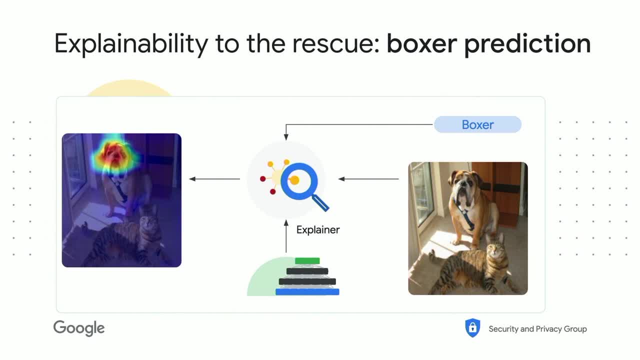 And if you do that correctly, you get something nice like this, which, as well, if you are trying to predict the boxer from this image using that model- and that's a true example from a ResNet model- then you get this nice heat map. 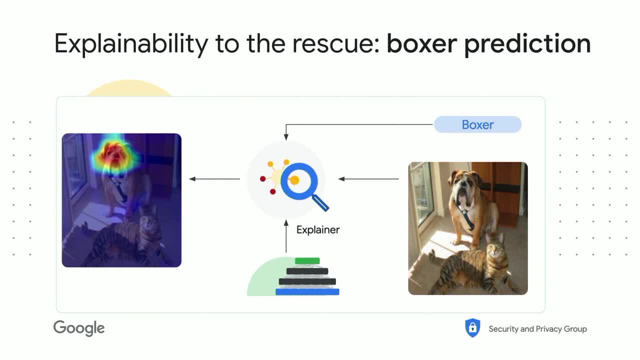 which we call leakage map later on for traces. That basically highlights that. well, it mostly focuses attention on the face of the boxer. So we have some confidence at least that the model is looking at the right part of the images to make its decision. 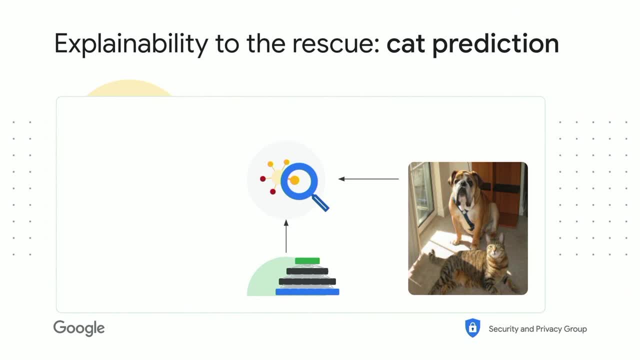 We can confirm that by doing the same thing for the cat right, Which we would say: hey, explainer, take the same image, take the same model. but now tell me why you came up with the idea of a cat, And this time it's looking at the body of the cat. 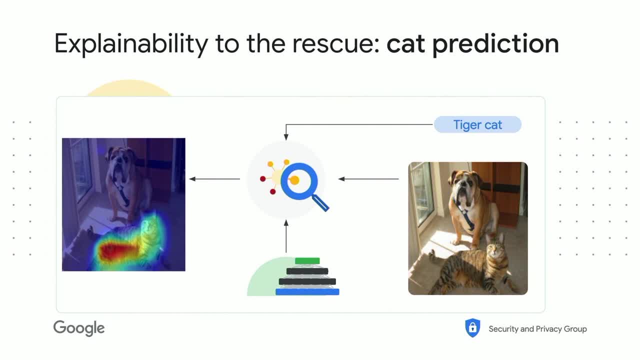 And because it says a tiger cat, it's looking at the stripe. So far, so good. That seems okay. So we are fairly confident that the model is actually working as intended, right? Here's an example where actually this type of technique. 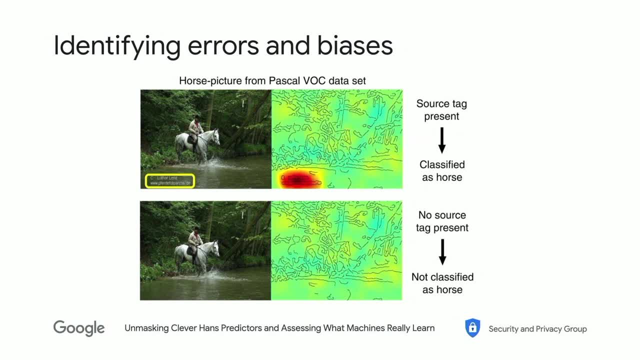 were used to find biases. Very, very early on there was this very famous data set for images called the Pascal vocabulary right Voc data set. And early on this data set has this interesting feature that for horses, as I think one in five had, 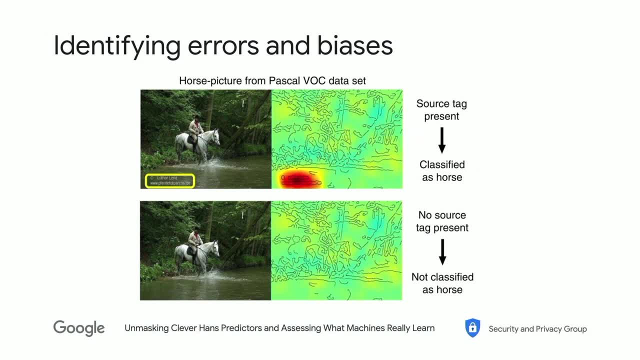 a text box on the lower left, And what happened was that the machine learning was predicting there is a horse, not because there was a horse in the image, but just because there was a box, And so that was very interesting. It was a biases. 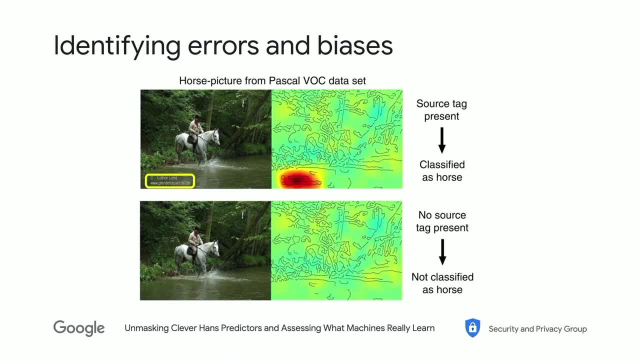 which were due to the fact that the image had a statistical discriminator which was easier to learn- there is a box or not- rather than learning the shape of the horse. This was basically the initial major success, I believe, for this type of explanation. 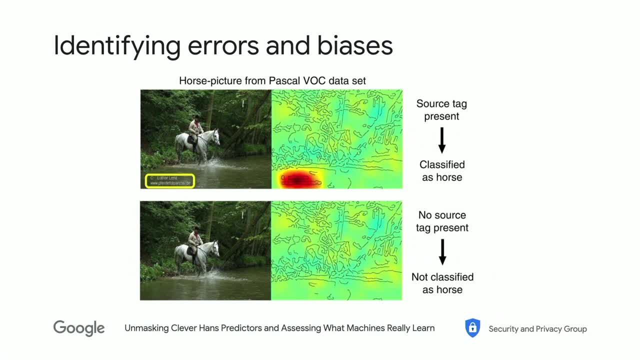 It was done into a paper called Unmasking Clever Hands Predictors and Assessing What Machine Learning Really Learns, which was published in Nature. You can, I believe the paper is widely available, not even without the paywall, so you can check it out. 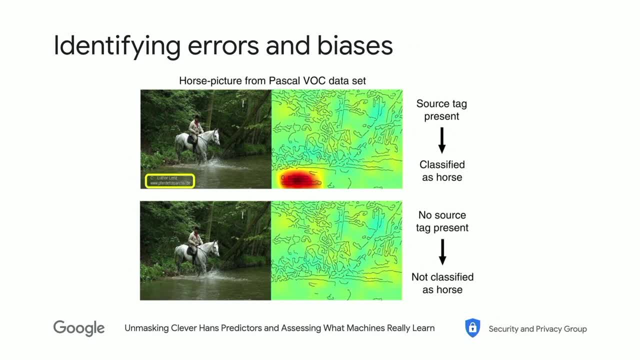 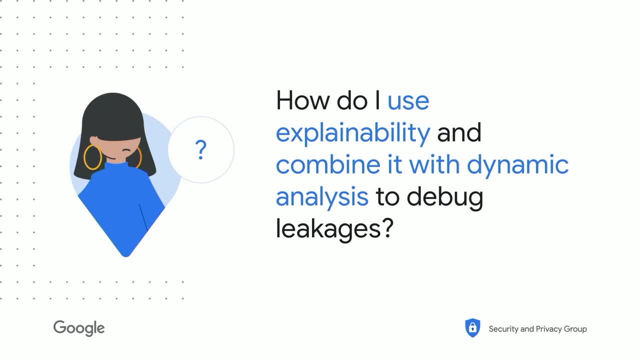 if you're interested into the origin of explainability. So that tells you how we do explainability. but of course, now the question becomes: okay, how do we use that and how we combine it with dynamic analytics to do what we wanted to do? 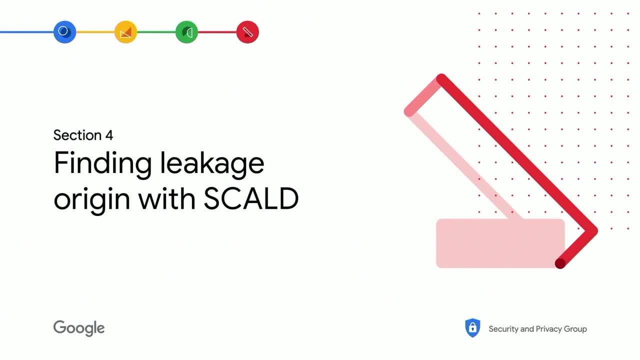 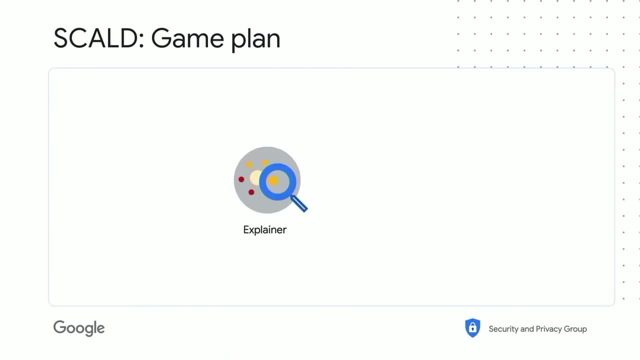 which is find where the leakage comes from. Well, this is where Skold comes into play. This is our debugging tool, which is written in Python, And so the game plan we have for Skold is well. start with an explainer. 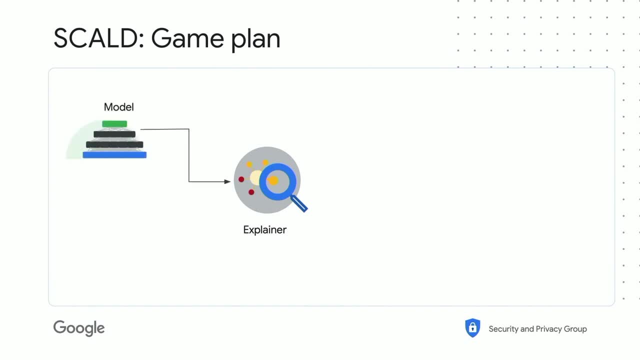 of course, and we're going to do very similarly, we're going to fill in the model which is our train model we see earlier, and the traces and the prediction for the traces. So we only keep the traces and prediction, which were correct. 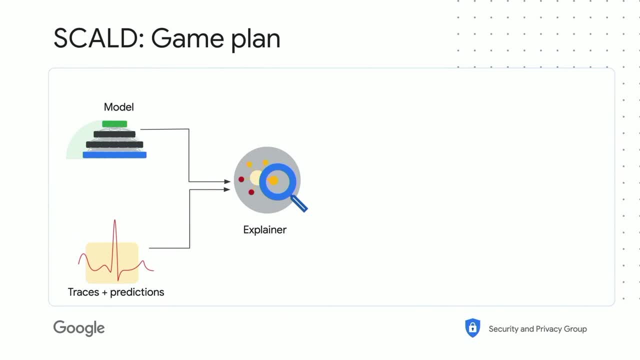 because we're interested in. why is the model correctly predicted, given the output of the biting? And then that's going to give us a leakage map. Of course it's 1D this time because it's a trace. It's not 2D like the images. 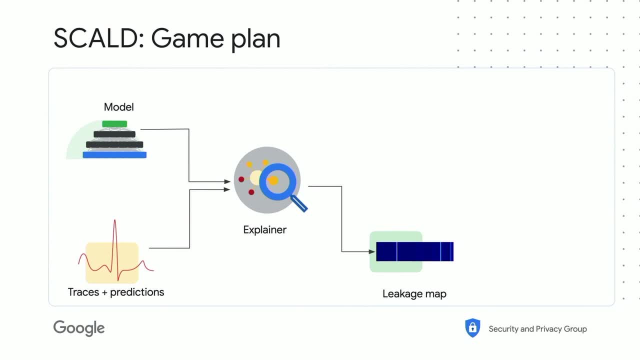 so that's what the leakage map is, And so basically, our hope is that the silent point into the leakage map will correlate with the code of that. But if you have a leakage map, you just know temporarily where it is. 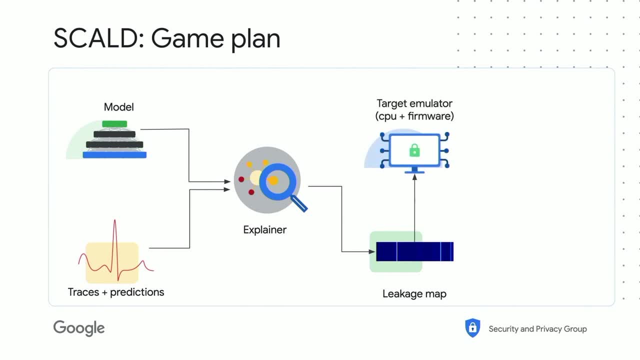 it doesn't tell you which instruction it is, So we need a different, a second piece of code, which is where the dynamic execution comes in, which is a target emulator. So, if you remember, the target is the code running on a given hardware. 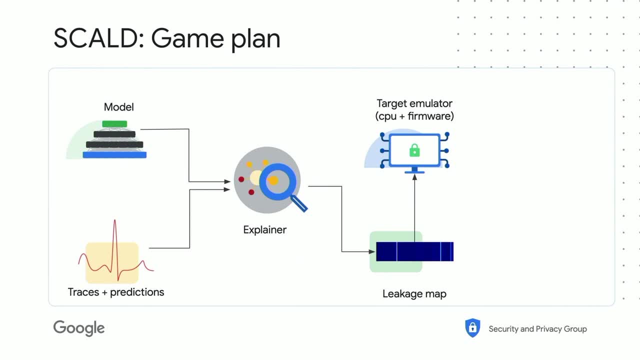 So for us it's TinyRS running on an SMTF4. And so what happens is it's going to take the leakage map and then it's going to execute the target and basically based on that and we're going to get the execution timing. 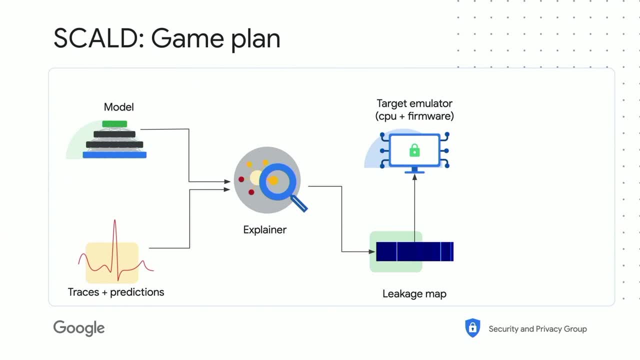 and we'll be able to correlate to know what execution was executed in which part of the traces. We're going to glue everything together and use debug symbol and you should be able to get annotated code with the leakage map and say: 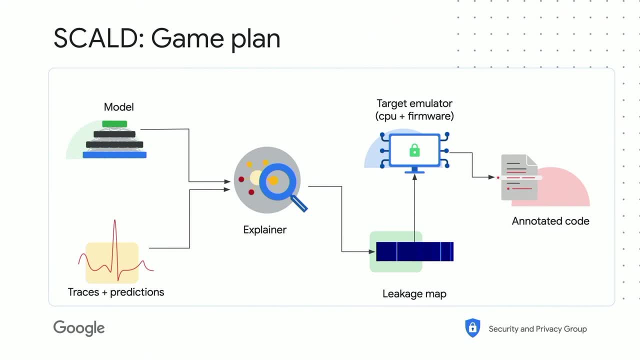 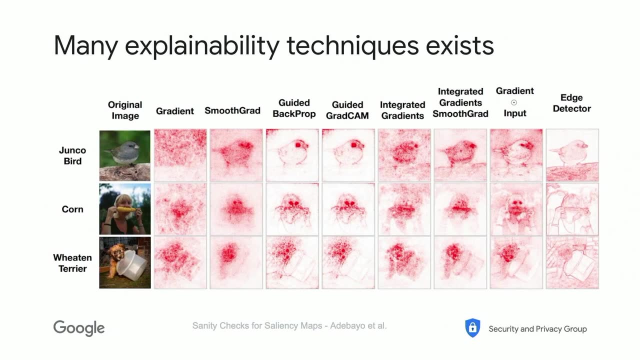 this is the line, the code line, which is the most likely to leak. Okay, So how do we get there? The first thing we had to choose is what type of explanation technique we should use, So we started by that. 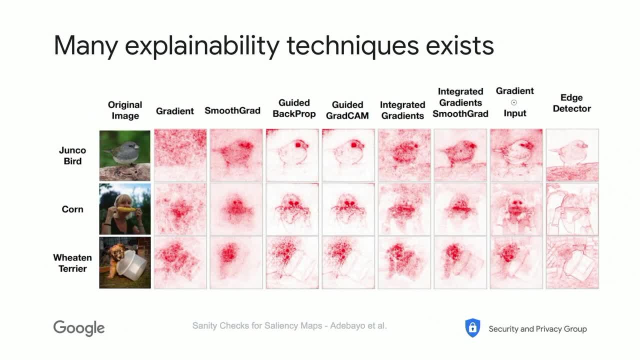 right, We need some explanation. So there is a ton of them. Here is some of them which were developed and you can see you get more or less a defined images or a defined output, So one we do use. 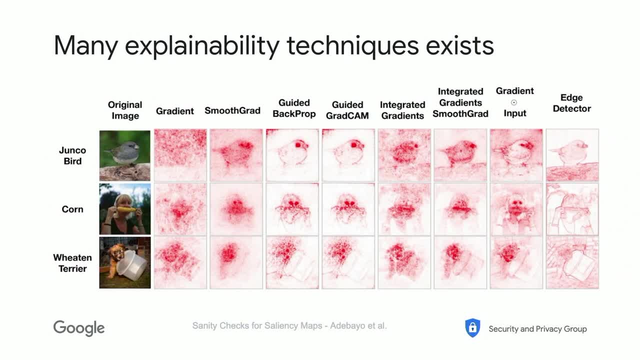 out of those is the one in the middle, which is a guided gradient, grad cam, which is actually. we use grad cam plus plus, which is a improved version because it's one of the most well-defined. We do also use something. 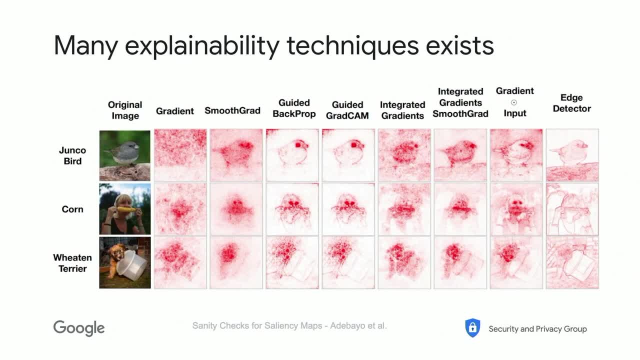 which is not displayed here, that I will cover later on- which is the activation map, which is literally just looking at the output of the first layer. So now that we know there are a ton of techniques, the question is: how do we choose the best one? 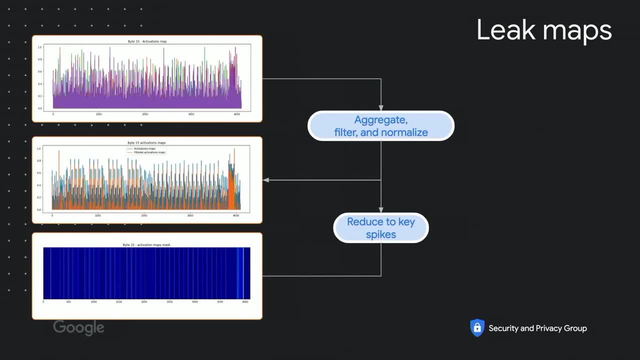 for our job right? And the answer is we have to benchmark them. So the way we benchmark them is we take every explanation we get for all the traces we get. So we use I don't know four, five, six thousand traces. 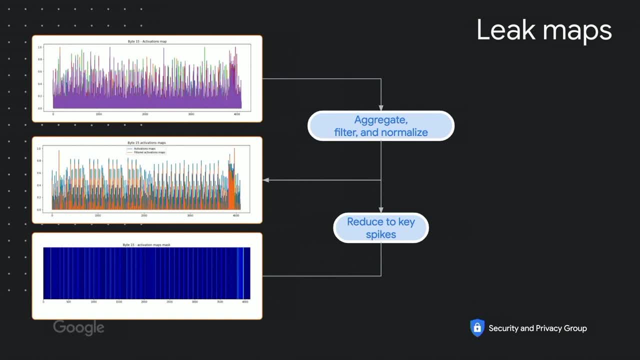 and for each of them we apply, we explain them. so we create a collection of them, as you can see on the top left of the slide, and then we combine them by either averaging them or summing them- it depends- and then we filter them. 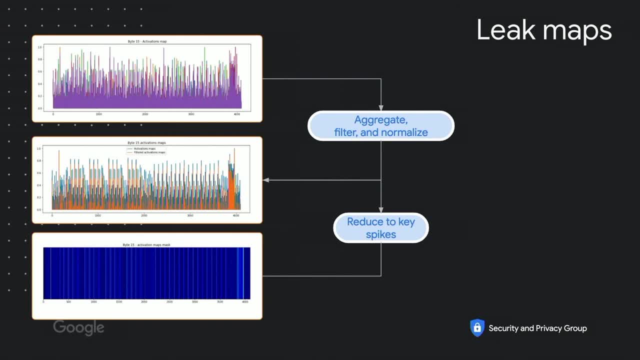 to only keep the spike. This is the orange part of the second boxes on the left. So this is what we call the average spike, and then we normalize between zero and one because we want to affect probability of what is the most important spike right. 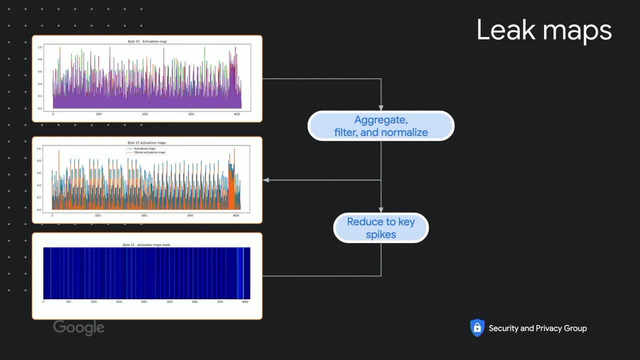 And then when you have done that and we have eliminated everything which is below the average plus one standard deviation, you get what we call the leakage map. and you can see, the leakage map generated here seems to have one initial spike at the beginning and then 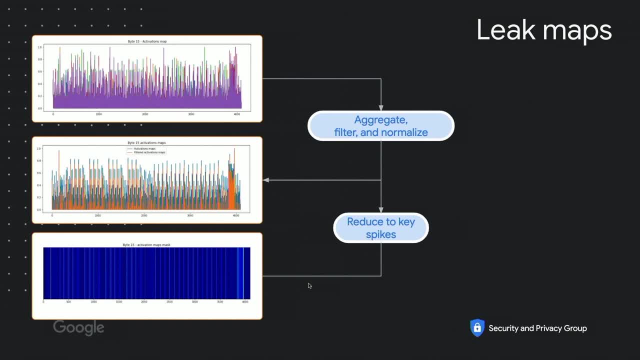 one larger spike at the end of the traces. Again, you can see that we have one initial spike at the beginning of the first round. Actually, we think that for this demo I cut it a little bit too early. I should probably have taken. 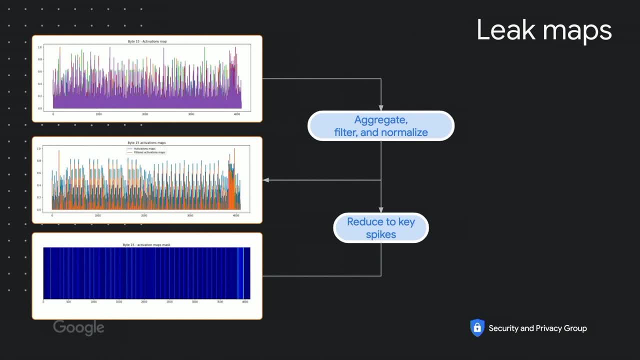 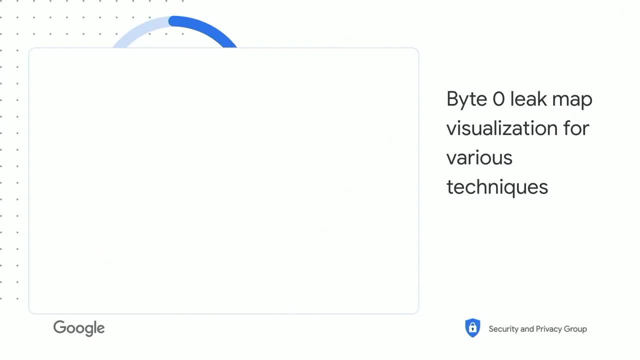 6,000 or 8,000 points, so we might miss the end of it, but suffice to say that for this byte it seems that we have one input and one output, right, So the thing we can do is we can generate. 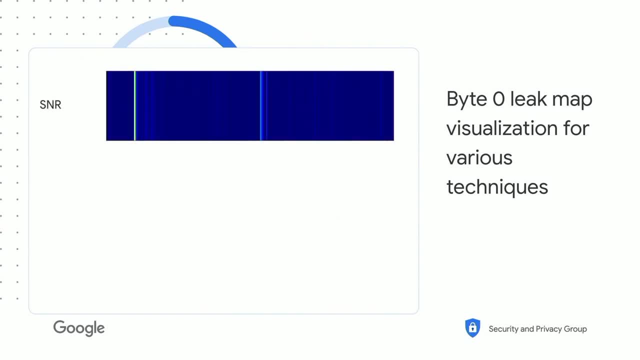 those heat maps for various techniques. So the first technique we use is the SNR right, The signal to noise ratio. This is not the deep learning technique. This is a very old technique which was developed actually to do traditional side-channel attack. 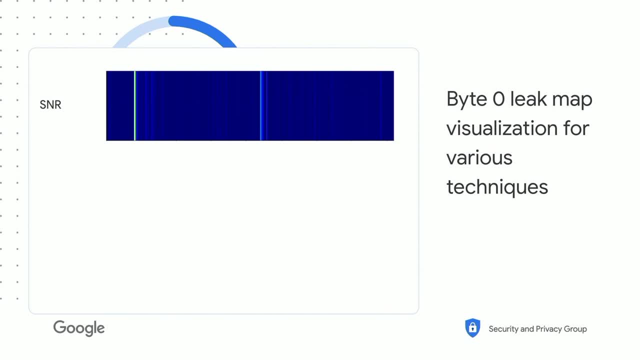 which is actually built in with Shippu Explorer, and we use that as a control. We are, we want to make sure that we use. we might also use it, by the way, but the idea is, this is SNR to noise ratio. 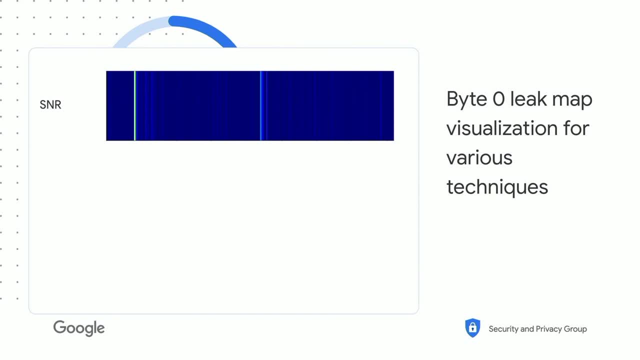 This is a standard technique where you look at, given some assumption, where is the spike, where are some spikes? based on this notion of where is the most discriminative part of the trace? This seems to be. this is four by zero, something at the beginning. 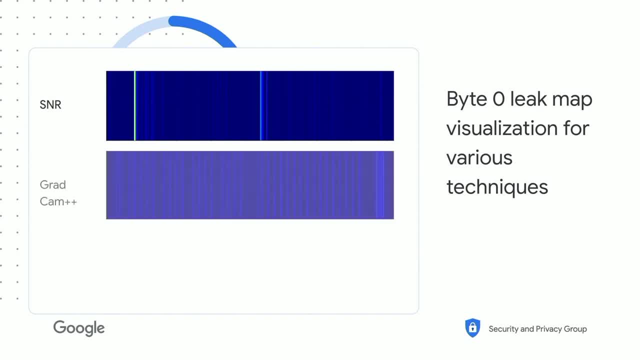 and something in the middle, and then nothing. Then we have the GradCAM++. As I said, the GradCAM is this idea that we use the integrated gradient and we compute some sort of inverted model where we use a gradient to see how it flows from. 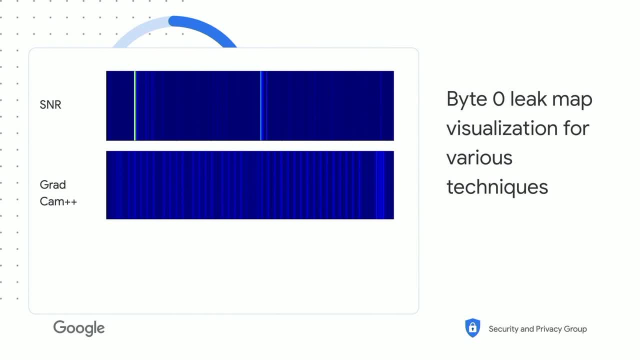 the input, the output, back to some of the layers, In our case the initial layer, because we want to look at each point individually and you get a very, very different map. We already know that one of them will be more correct than the other one. 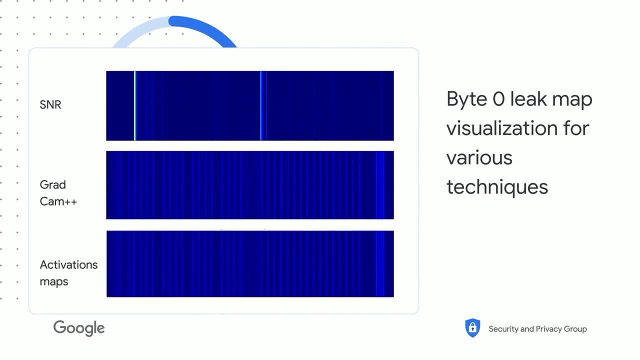 Then a third technique we use is called the activation map. The activation map is basically you do your prediction and then you look at what were the value of the each of the different, how much each neuron did fire, Because we use the lowest bottom layers and these layers 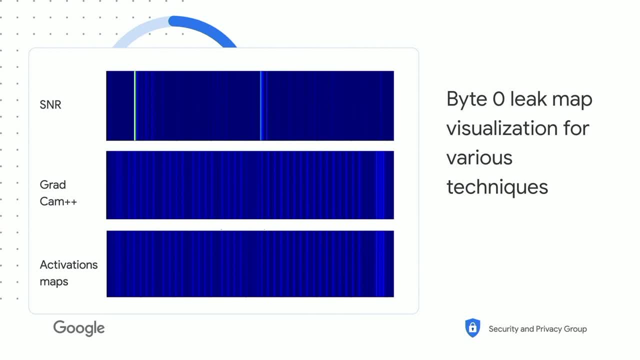 is the size of the trace, how much it did fire. What you can see here is it's mostly identical when filtered to the GradCAM++. Both of them are somewhat identical, so we expect them to be performing roughly the same. How do we evaluate? 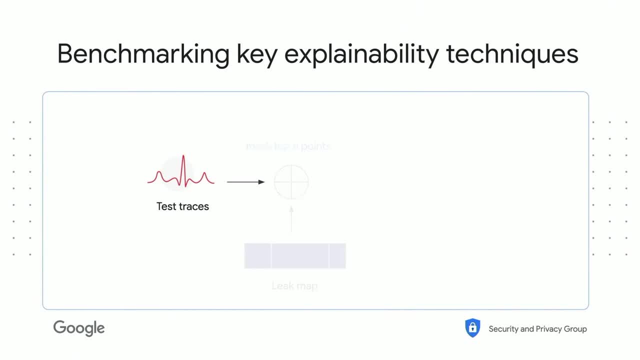 the quality of this. The idea is very simple. We have our test traces and we have our leak map. What we can do is we can decide to suppress, which is basically putting the point to minus one. The machine learning normalizes between two points. 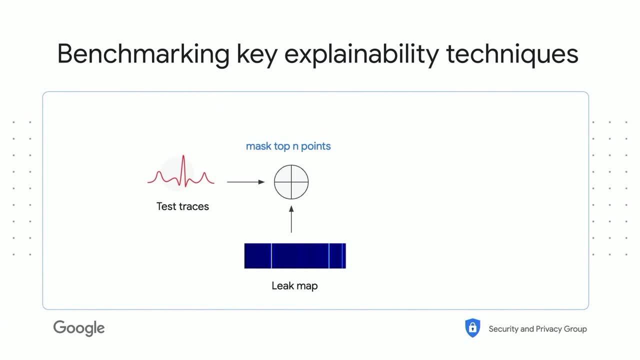 and then we remove them. So what we can do is we can take what are the four, six, seven, eight, 20 points. after that become meaningless. But the first top point- that are reported by the leak map, suppress them from the traces. 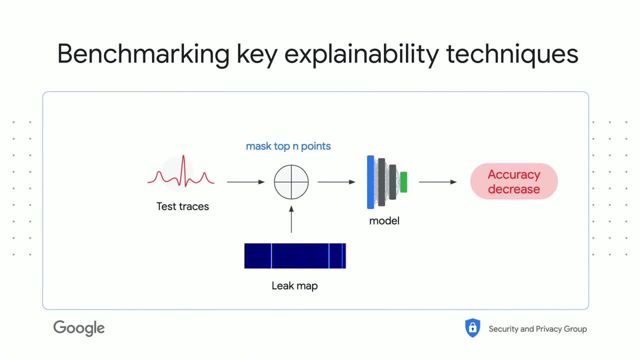 feed them again to the machine learning model and look at how much the accuracy did decrease. So basically what we'll tell us is if those points are important for the machine learning to the predictions. you care about everything, so you'll see always a decrease, but it might not be. 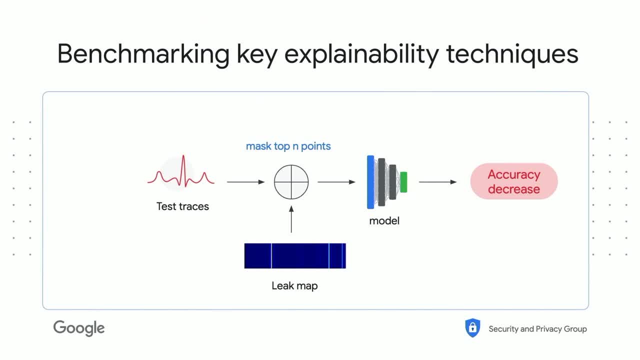 as drastic. So now the question becomes: if you fix the number of points, how much of a sharp decrease we do The ones who decrease the most? the accuracy will be the technique which is the most predictive of the leakage. That's the technique. 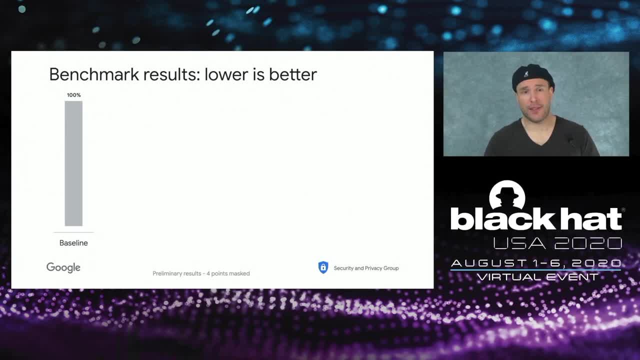 we're using and how we do benchmark our explainability technique. So baseline, as I mentioned, is 100%, because we only kept, as I said, we can look at each of them. So first thing we can look at is, as I said, signal to noise ratio. 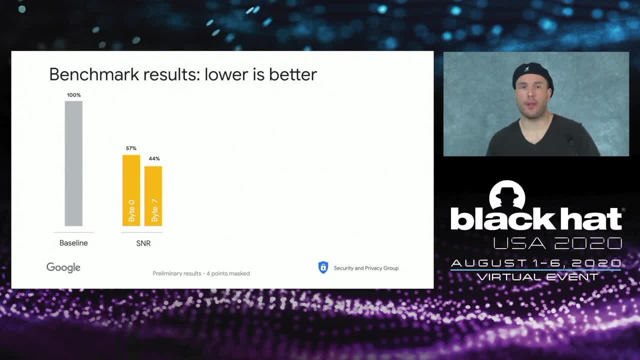 and in that case, on byte zero, the drop of accuracy for four points is 57- is dropped to 57%, which means we have a 43% reduction, So almost half. So in four points- there are four points, the SNR top four points. 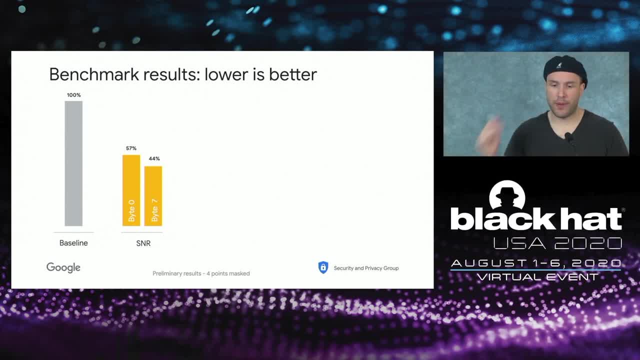 are responsible for about 50% of the accuracy of the model. So it gives you an idea that these are really where the leakage are coming from. Similarly fairly consistent with byte seven, where it's even deeper: 44%. Now, if we look at activation map, 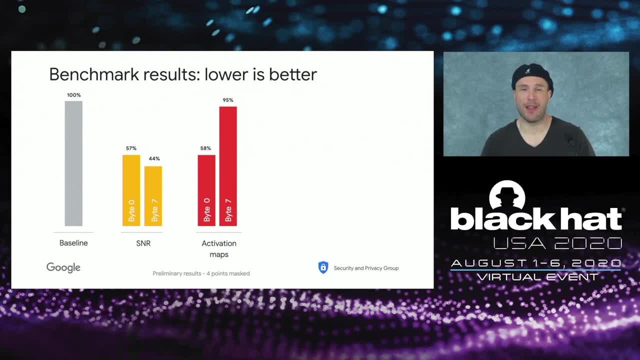 that's where we start to be really sad. if we were very sad, The activation map performed really worse than that. So about the same for byte zero, but then for byte seven. what the leakage? the activation map return is not predictive at all, or at least not. 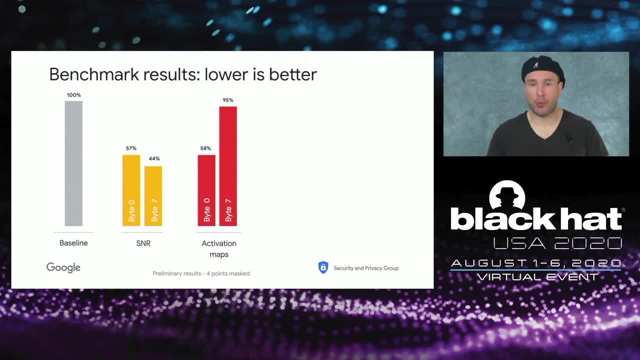 given our benchmark. So we're hoping that GradCAM++, which came as one of the- not the latest, but one of the most well used one and is supposed to be really good, at least work really well for images, will work well for us. The thing is. 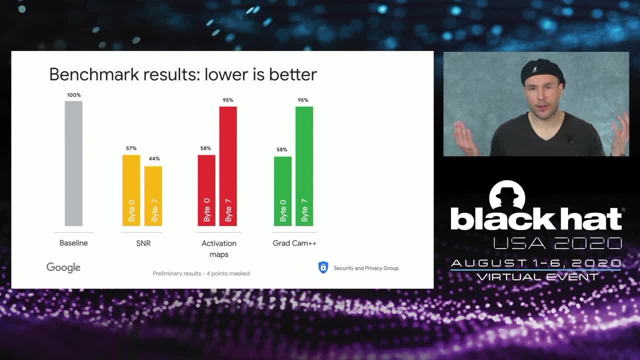 if you remember, I showed you they are almost the same leakage map, so you get the same result. I mean, that's consistent, that's good, but the numbers are really, really bad. We still, again, do not get the hypothesis which we know are not as accurate. 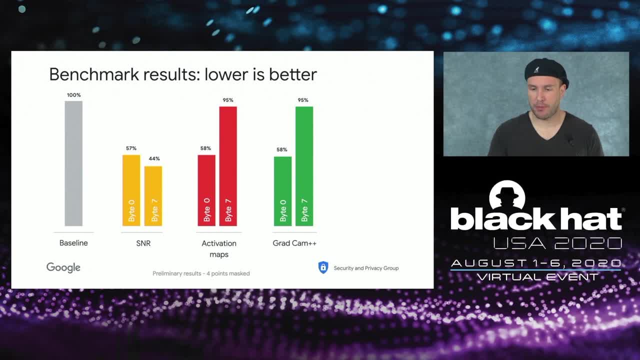 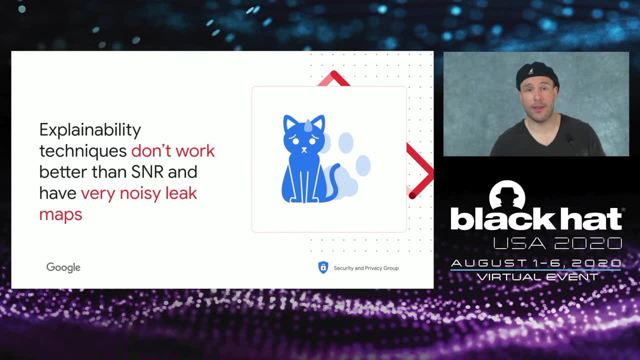 as the machine learning one, because they use the hamming model, if you want to be precise. So we were really sad because- and it took us a while to figure out what to do- because actually the explaining technique we wanted to do did not work and the SNR. 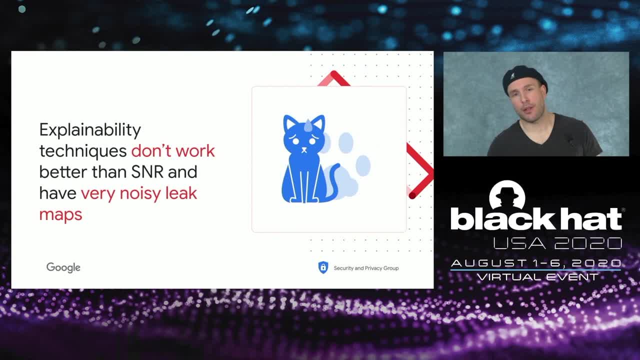 than the SNR and also, as you have seen, we could have said: well, but they are cleaner and they're not. They also have a ton of stride, so they're not very informative either. So it took us quite a bit of iteration back and forth. 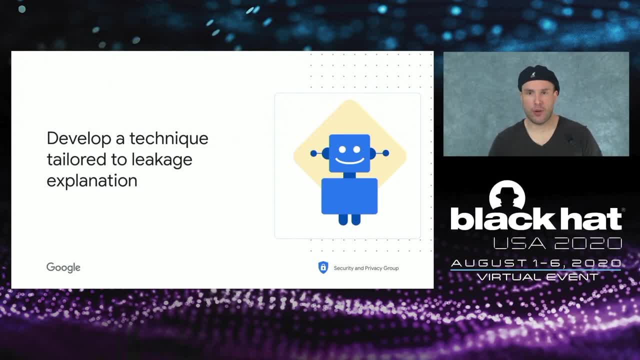 and then we ended up deciding that we need to create something which is a little bit more tailored to what we wanted to do. So the reason why that might work- and I know you might be skeptical that we can't come up with yet another technique- and why it would be better: 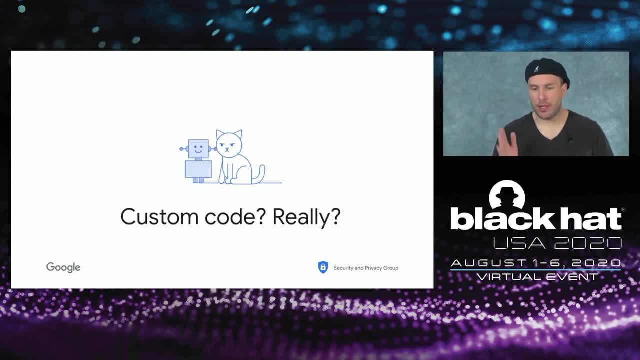 so the reason why it might be working better is because usually the machine learning technique used for explainability focuses on the highest level features. so the world of the neural network, to get more of this understanding. and what they do is they stretch, because the neural network is like a 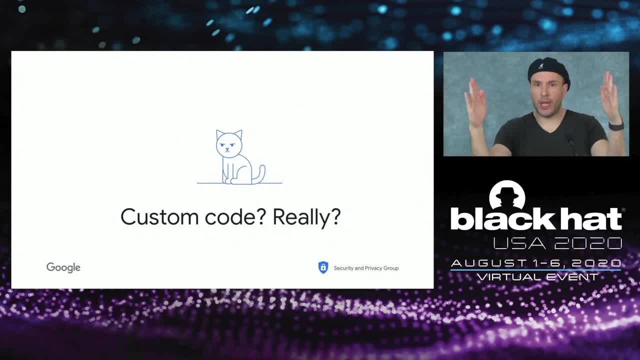 pyramid right, so the upper layer are smaller in width. so you have to- if you want to put it back to the trace, you have to stretch them out. We don't want to do that because it basically creates inaccuracy. so we try to do the explanation. 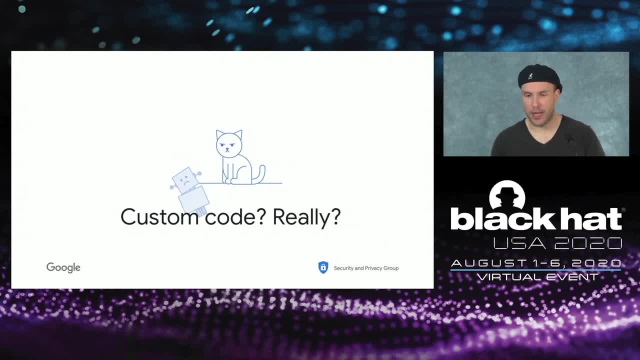 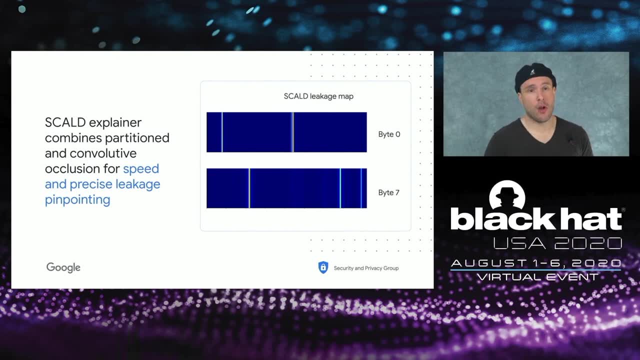 at the lowest layer, it doesn't work right, as we saw. So the idea and actually use one of the oldest techniques, but revisit them to make it a little bit more precise, which is using occlusion. The problem with occlusion is that an occlusion. 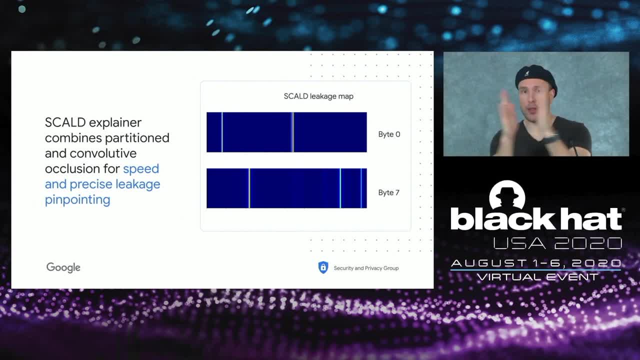 is basically you are removing part of the trace and you're scaling it that way. The problem with that is, of course, it doesn't take into account non-linearity. so to combat that, we came up with a novel version which is basically combining this type of occlusion. 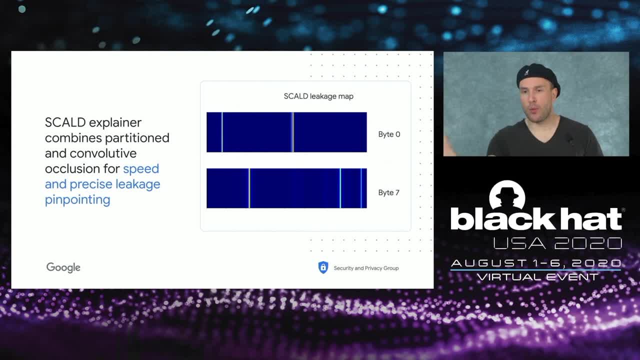 by block, with a convolutive occlusion, which is basically using windows and then convolving the squares to get some sort of back of non-linearity over a large region or small region, like a set of small regions, And so what you end up with? 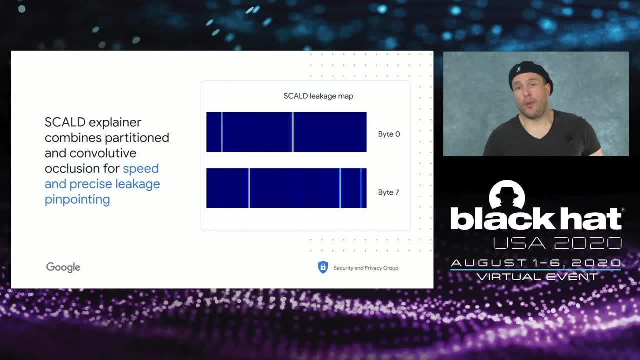 are the maps you can see here. So the first thing about those maps, just visually, is they look very clean right. There are only very few spikes, so that's good If they work, it's very clear where the leakage comes from. The other thing: 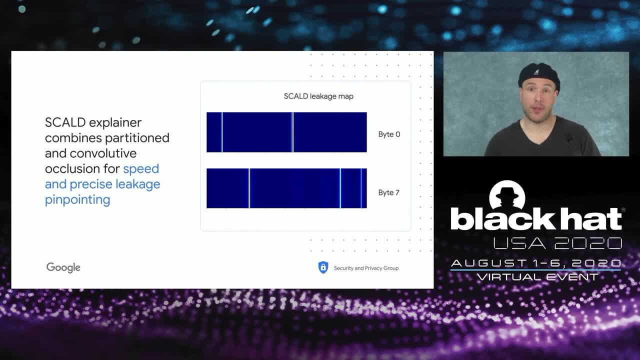 which is very encouraging is leakage before the byte 7.. Of course, the algorithm processes one after each other. it's not using any kind of themed or vectorized operation. so that's what we expect. We expect it to do: one, then the next, then the next. 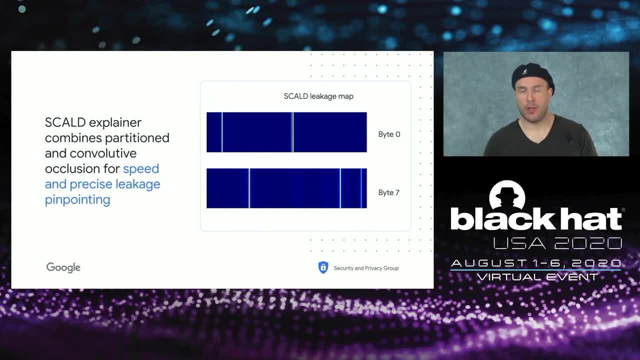 then the next. so we're pretty good, confident that it actually makes sense. It also interestingly shows you that port of byte 7 actually is really close to the end of the traces, which explains why, as I told you earlier, I might have the trace to be too short. 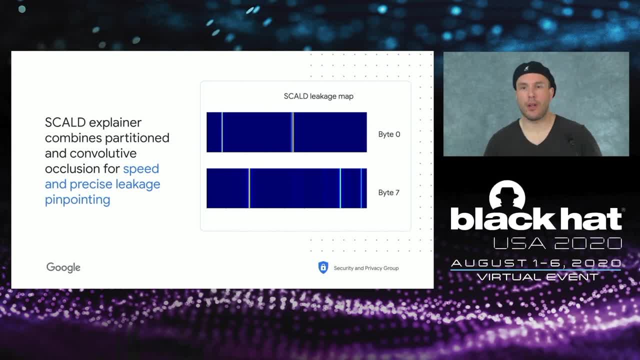 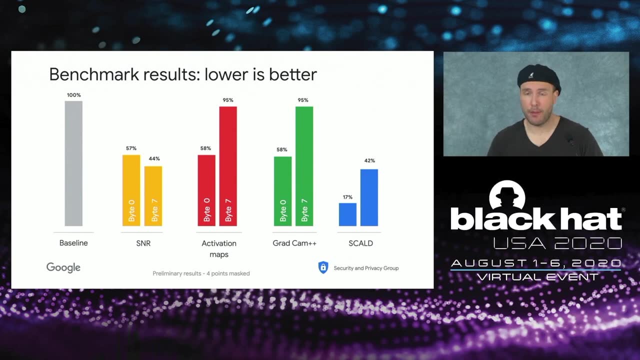 or even byte 13 and so forth, because we already have the limit for byte 7. that's why we did cut here and so, yeah, it looks good. so now we can benchmark it and the answer is how good it is? the answer is: pretty good, it's. 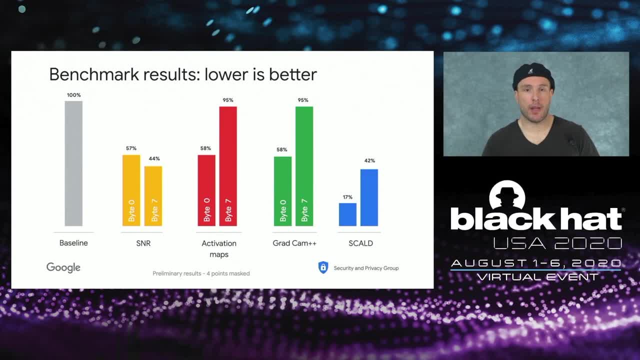 way better for byte 0: 17%. so way, significantly better than anything else. and for byte 7 it is better than SNR, to be honest and to predict that, that's for 4 points when you look at 5,, 6,, 7,. 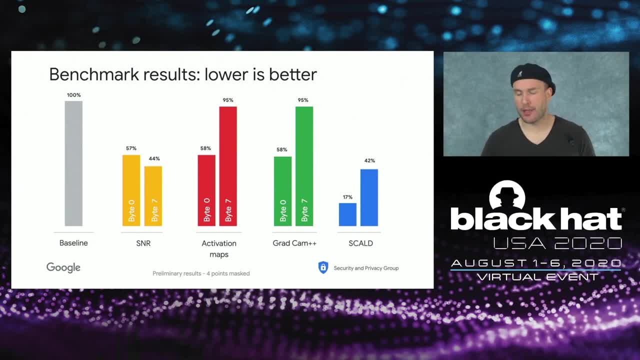 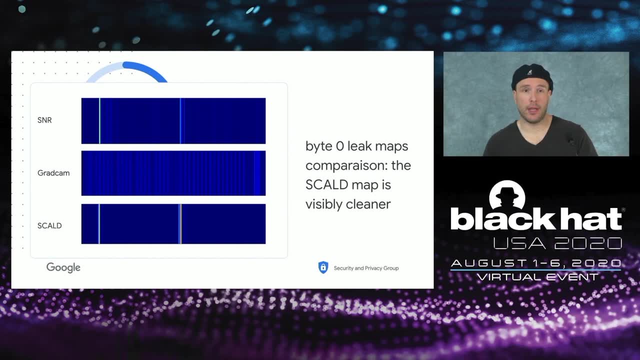 8 points. sometimes one goes above the other, but overall Skoll performs better. so we have a technique now which works really good, really well, and if you compare the quality of the traces, the first thing you will notice is actually the Skoll traces is very similar. 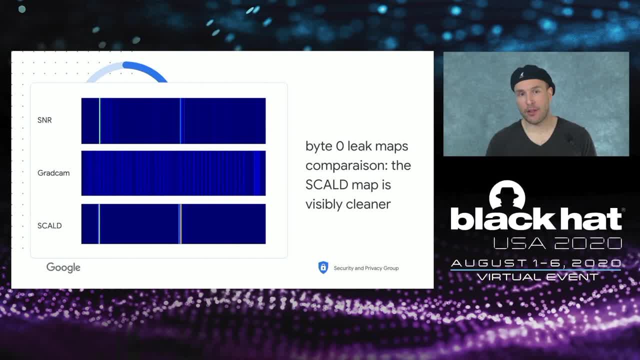 to the SNR, one for byte 0, except the SNR is gone. so now we have three, two very clean parallel traces. that we know is responsible for most of the leakage, which is good. also, Skoll believes the it might not be very visible on the slide. 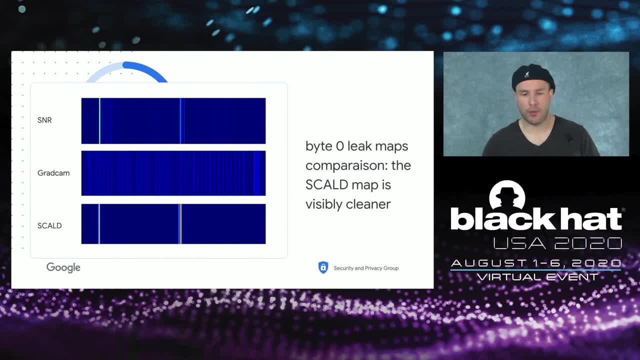 but there is a red bar in the middle. so Skoll believes the second spike is more important than the first one, whereas for the SNR that's the reverse. so interesting the differences between the two. and in the middle I put GradCAM++ and you can see. 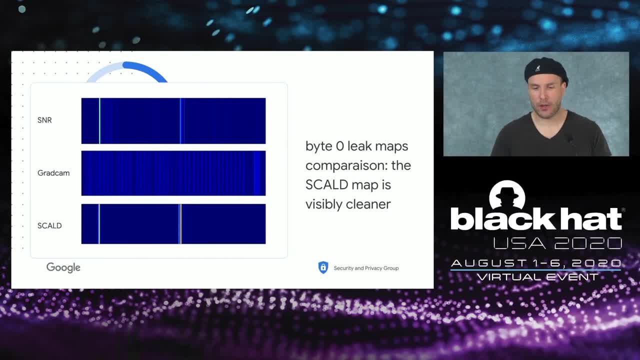 we have confidence. we are finding almost the same places. so we are confident it actually makes sense. at least it actually makes sense from even a statistical analysis. so that gives us a lot of confidence that it's the right technique for the job. so now we're back on track. 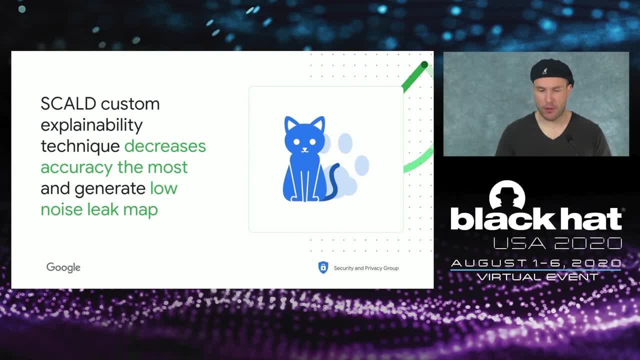 we have a technique which decreases accuracy the most and has very, very low noise, so when we use it to explain the code, the developer only has a few places to look at, which is really good. so now, how do we go from the leakage map to the code? 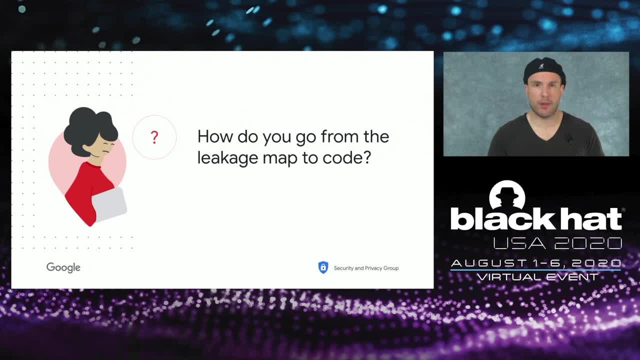 and this is where I'm going to be a little bit hand wavy, because this is a part of the code we are still actually working on and I don't have a slide to show you the end result, but I will explain you where we are at. 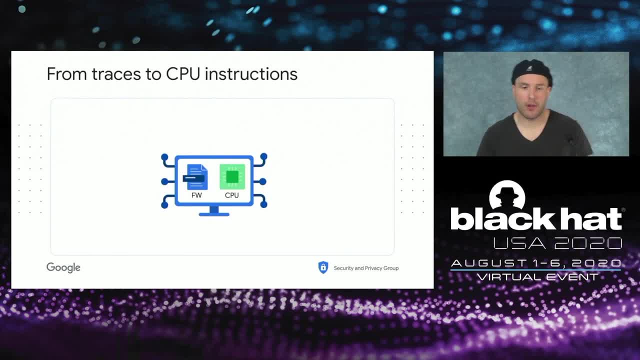 and I can show you where we are. so the idea is how we go. the first thing we need to do is, as I said, you go from the traces to CPU instruction. so CPU instruction is going to depend on two things. the first thing is what type of CPU. 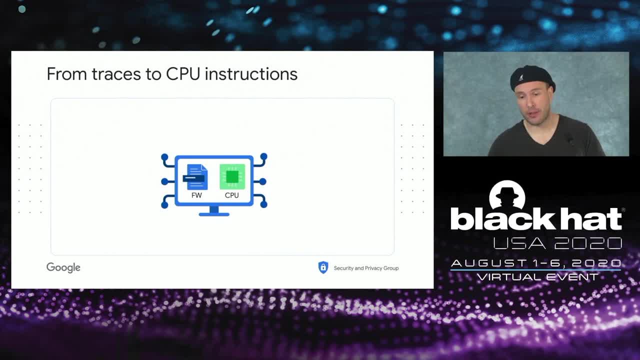 so we need to know for each instruction how many cycles it takes. then we need the firmware, which is basically the compiled version of the code which tells us which instructions are executed. we need to fit the leak map which tells us which points are important for us, and we also need 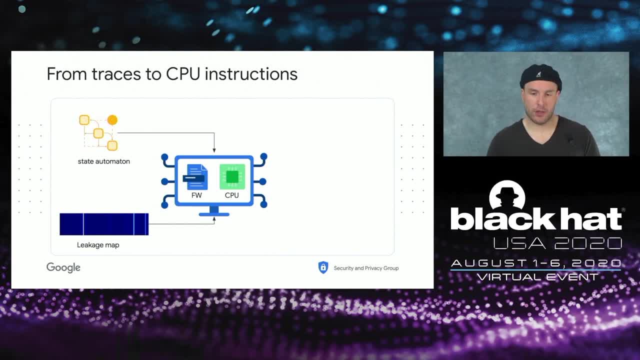 to have a state automaton who instruments the emulator to be able to reproduce the encryption, and so we can basically reconstruct what instructions were executed at which time and then map it back to the trace, which will tell you what point in time is important. so, with all 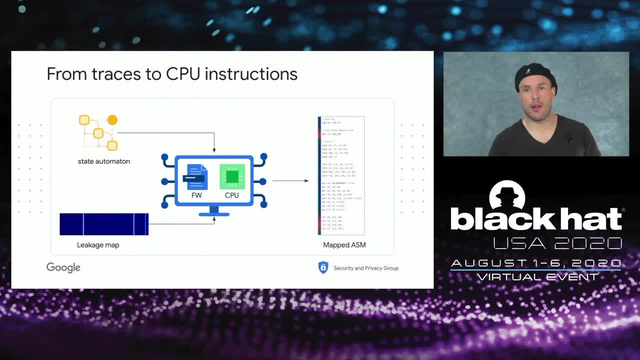 those things. what you get is you get a heat map of which CPU instructions are the most important. this is the part we are still actively developing, because we need to refine a little bit how our clock and program counter are implemented to be as accurate as possible. but this is. 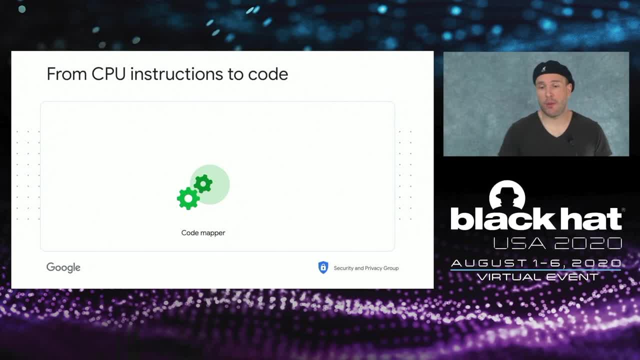 what it does, then what we need is: now we have assembly code, so we can probably end up there, worst case, but we want to go one step further, which is: can we go back from assembly code to C? and this is something which is well known in the security community. 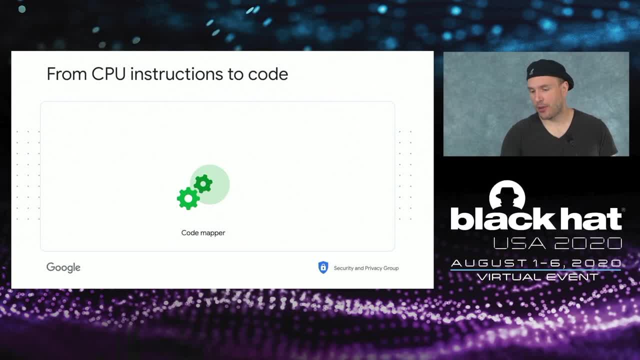 that's what is the bread and butter of reverse engineering. so there's a lot of product to do that. but essentially what you do is you take your ASM and then you take your debug code again. we're in the debugger setting white box, so we know what debug code. 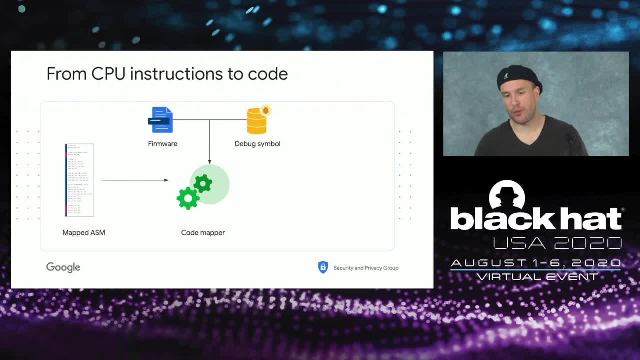 and then the debugger can easily go back from instruction to line of code thanks to those debug symbols. so from there it's fairly trivial to go back to the leak, to the leak code. so now we have the code alongside the heat map and hopefully, well then, now you know. 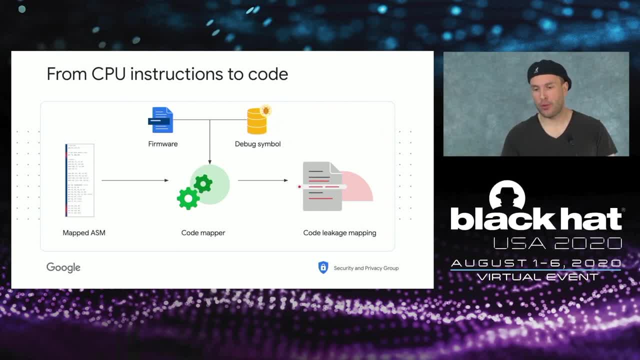 which line of code is causing the most leakage according to machine learning earlier. the machine learning explanation is very well correlated with the SNR. we believe it's also going to surprise the template attack which uses this kind of statistical ratio. so everything should fit together, I wish. 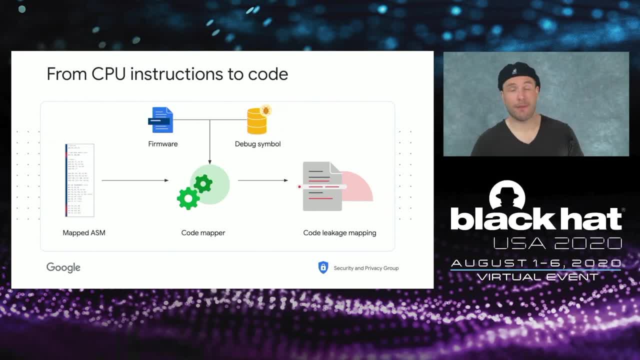 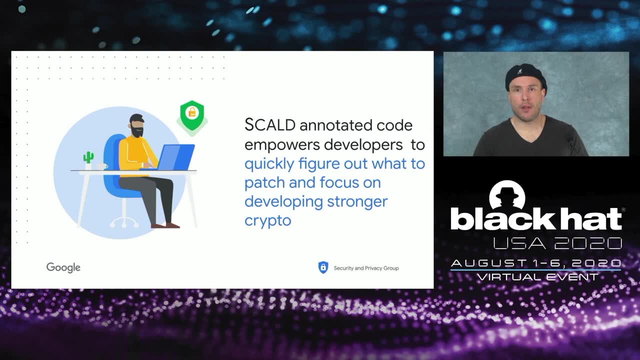 I would show you for 10 years the exact line, but, as I said at the time of recording July 14, we are not there yet. we are still refining it, so hopefully we get that by black hat all right. so the idea is that we can build. 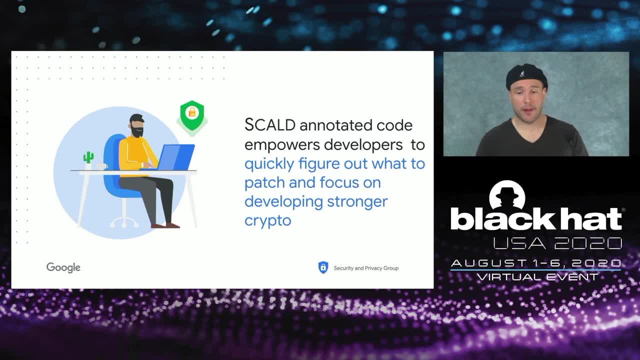 this tool, which is going to hopefully empower developers to quickly figure out what to patch and focus on developing stronger crypto more than how to do the size and attack and everything, and freeing up more time to focus on design and experimenting with new masking technique or protection or things like this. 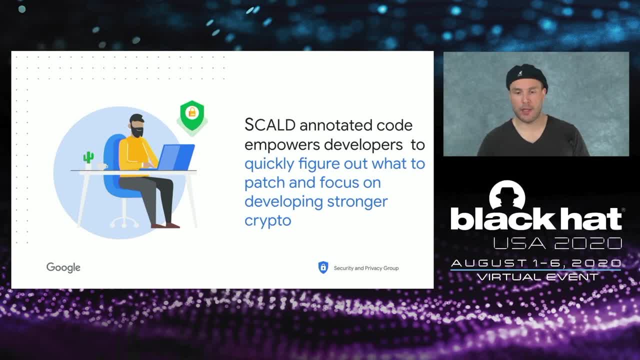 we are really excited to test it more and have a little bit more use cases for it and hopefully generalize. so far we are very hopeful it's going to do that and it's going to help us. the main benefit and takeaway from this talk should be that. 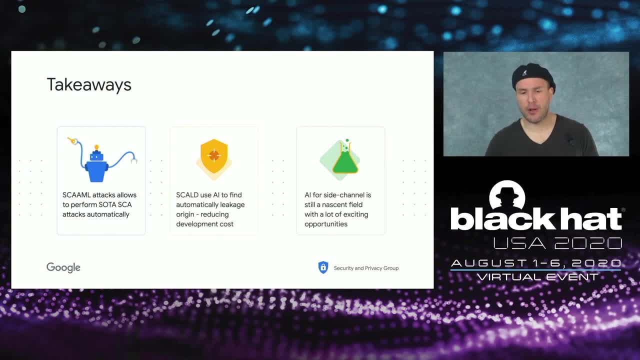 a. as we mentioned also last year, machine learning is a new is a way to perform state-of-the-art SCA attack automatically. it actually is changing how we approach a channel attack, because it's allowed to automate a lot of things and also it's able to do before. 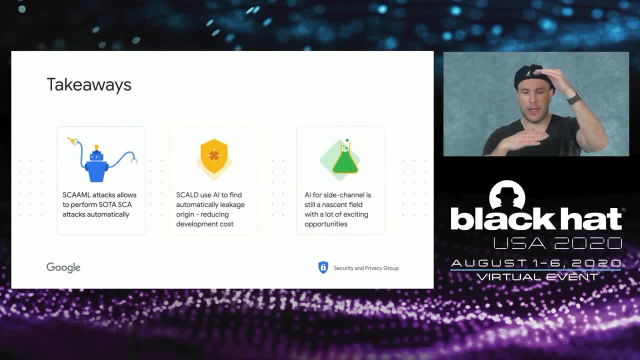 however, they also have- as I showed you with the leak- how the leak map actually aligns- that they are also finding the same type of stuff that you would find with SNR, plus more, so it's literally a upgrade. the second thing is we showed you in the middle of the talk, 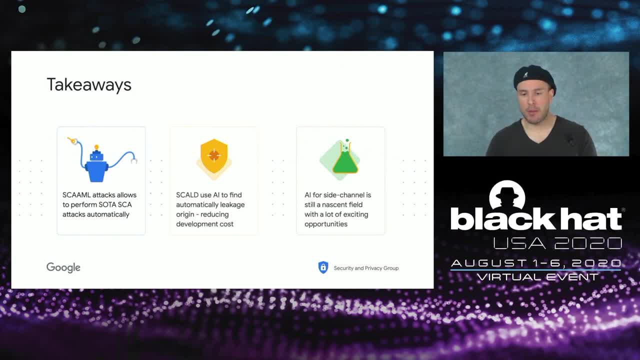 how we can actually combine this AI capability with dynamic execution to try to find leakage almost automatically and then helping reduce the development cost of secure hardware and hopefully it would help us to have more secure hardware through the world. and finally, there is a lot to be done. 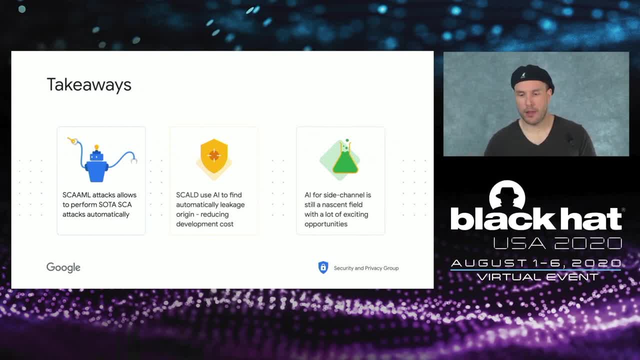 while this talk shows you a way to do it. we don't claim this is the best way, just a first step towards that idea. there was other research, by the way, I need to mention, who are exploring the same idea. some of them from the ANSI did some of this type of research. 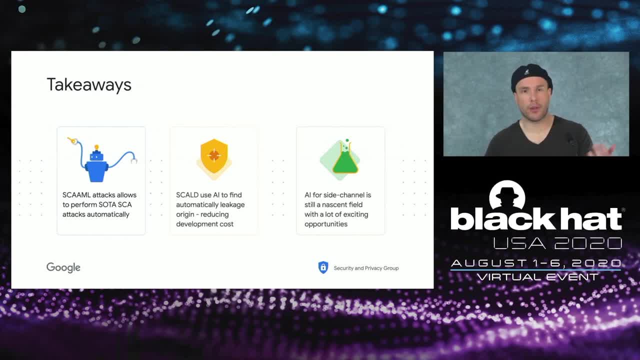 as well on how to use explainability. I don't think they went as far as us, but I think this idea is a community and it's a very active community. there is a lot of work to be done in the idea of combining alpha playing, AI for such an AI. 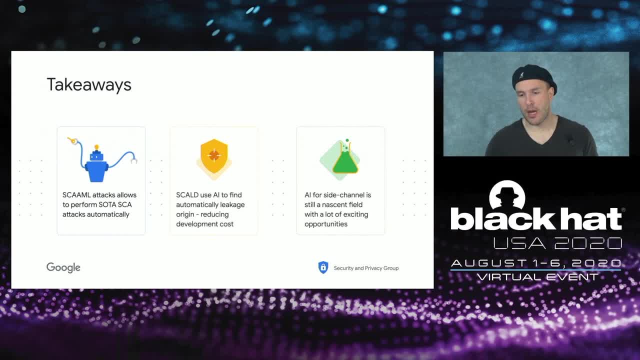 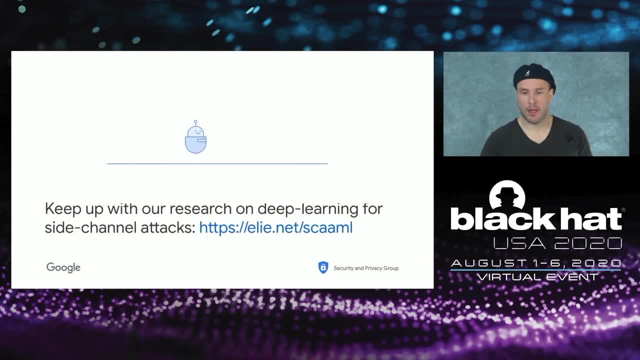 whether it's for improving attacks or improving defenses, and so we're really excited to see how this is going to turn out and have collaboration with as many people as we can so we can build the most secure hardware we can. thank you so much for attending this talk. 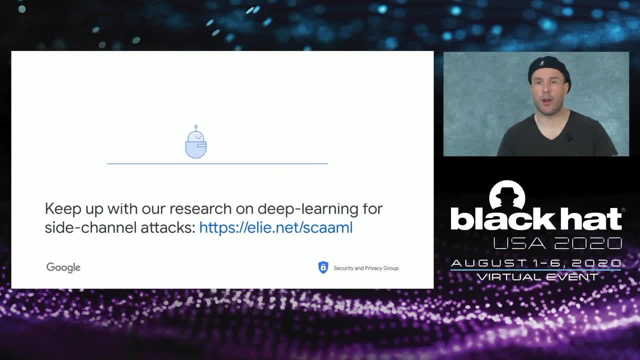 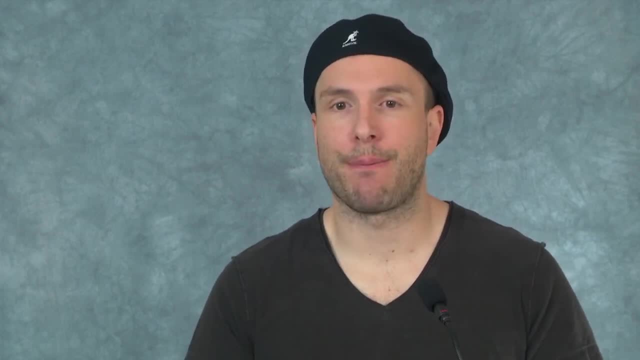 virtually. I hope you're safe at home and if you'd like to keep up with our research and be aware of new releases, you can always check out the website and you can also follow us on Twitter, where we try to post our updates. thank you so much. 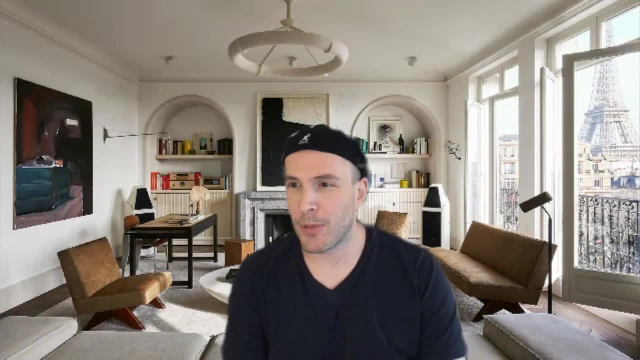 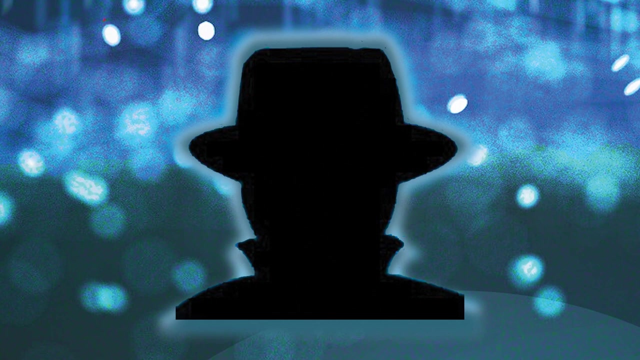 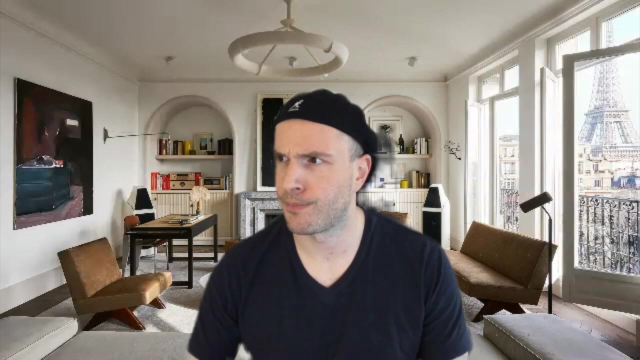 for attending and we'll see you next time. bye, bye, oh, I'm sorry. yes, it was. I apologize. I was saying thank you so much for you guys for attending the video, and can you guys? yes, no, you should be able to hear me. thank you so okay. 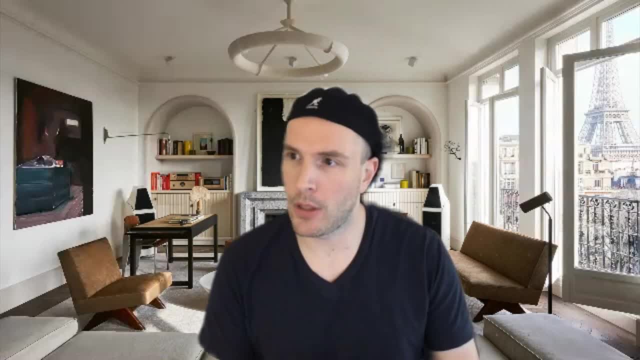 sorry, there was a a problem with the audio so I said thank you so much for attending. as you have seen, three weeks ago, so about three weeks ago, so we didn't get all the results in. I did add them to the, to the slide deck and, if you take the latest, 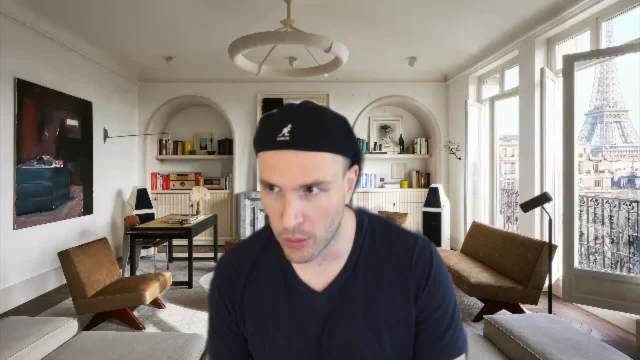 slide deck, you'll see that we actually did in the end using our tools code. the question was: which will we use? well, that's our own tool and we're going to make it available on github and you will be able to play with it and reproduce the research.